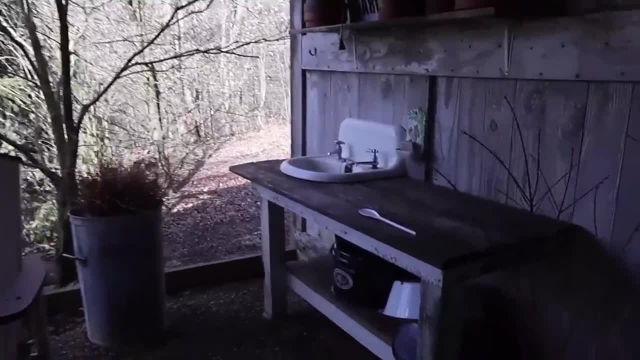 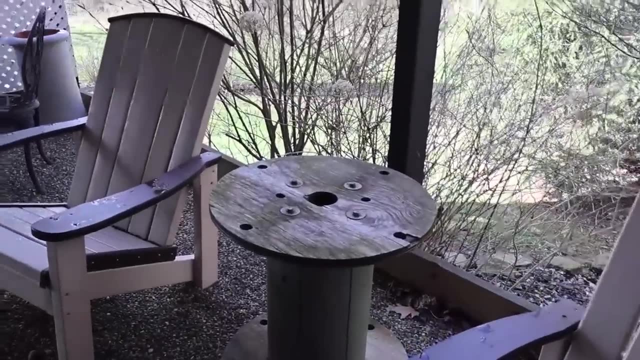 in. I like to do it outside and often I'll do it here on this bench. There's the spoon that I use to mix it with, or this little table here- spool table- and a little black table over there. I even have a light to work with if it's dark Sometimes during the winter. 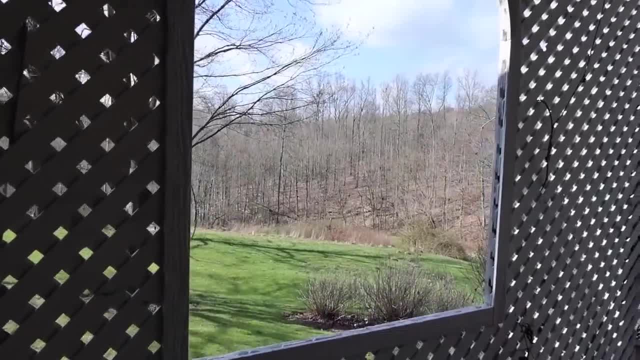 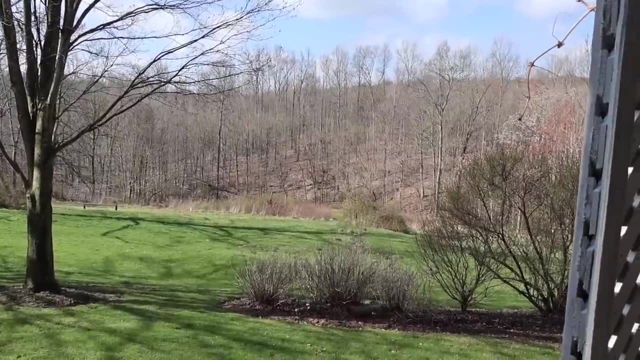 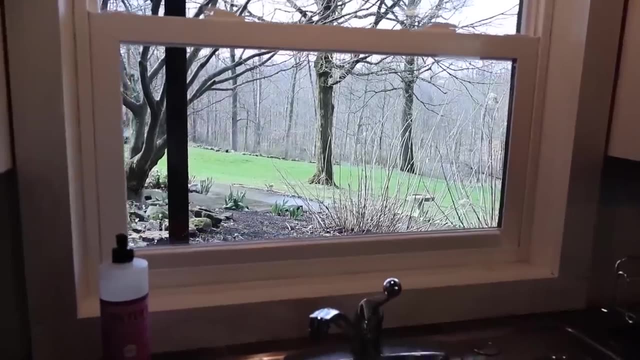 it's dark when I make soap And, of course, a morning like this is just beautiful to enjoy the sounds and the views. out here You might hear the phoebe singing Such a spring-like sound. As I'm mixing soap or washing dishes, I can watch little birds hop around on the 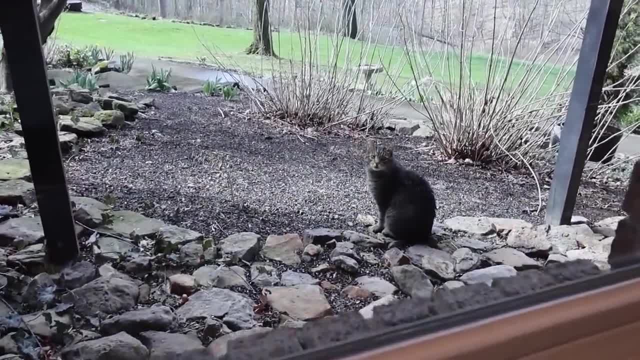 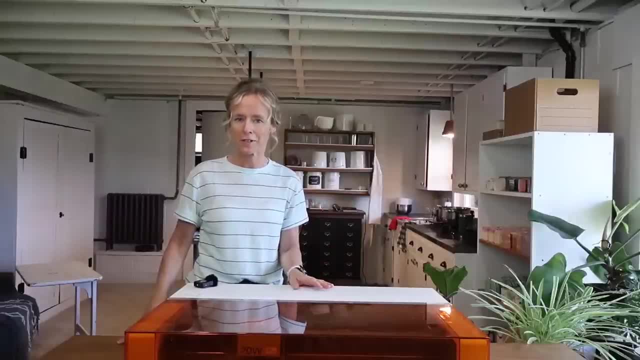 outside. The seeds that fall from the feeder above attracts them. Pretty sure there's none here now, So I'll be working on spring scented soaps in this video- one of my favorites- And of course, Lily of the Valley will be in this mix. You guys know how I feel about that one. 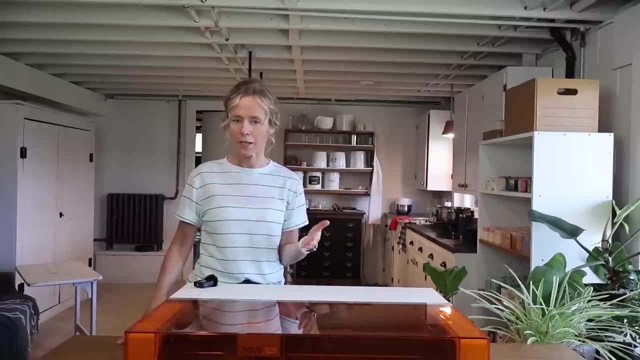 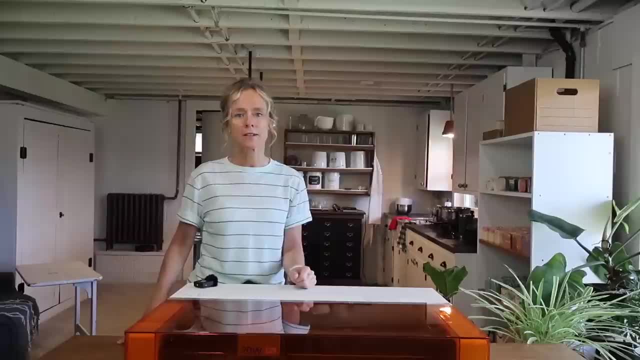 to try it out. I'm going to try it out, So stay tuned for that, But just follow along as I make soap. I'll probably explain a little bit as I go, but for the most part I just want this to be a relaxing video. If you're like me, you sometimes need that, In fact. 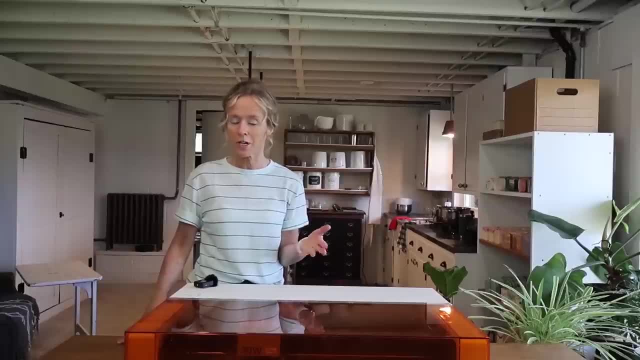 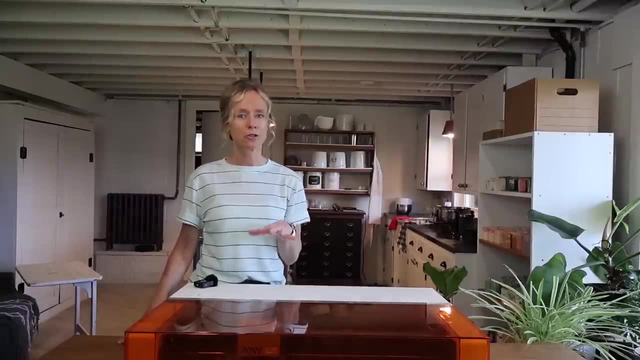 I sometimes use soap making videos to fall asleep to. I know it sounds weird, but to me it's just so satisfying and relaxing and peaceful to just watch someone make soap. I can't wait to show you the labels that MB made. They turned out so cute. Let's get right. 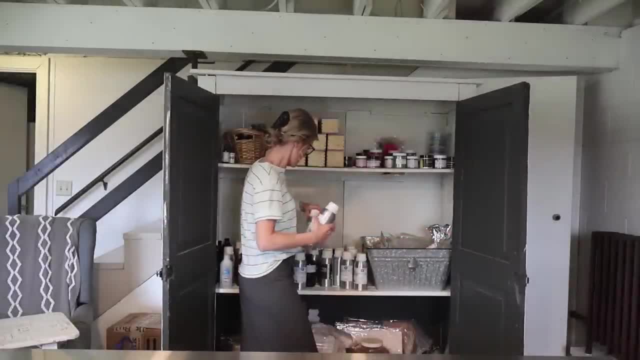 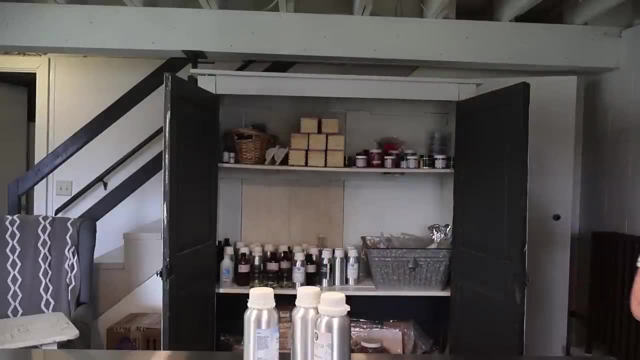 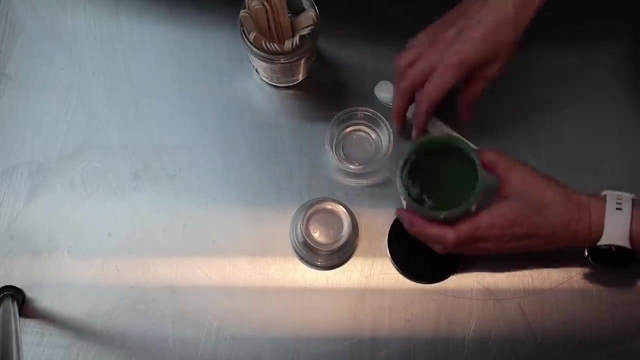 into it. I have learned with making soap: you cannot be too prepared, like just to get everything ready beforehand before you mix that lye and water together and melt your oils. So that's what I'm doing here is just gathering everything I need for today, including all of my oils, mica powders, and I have little containers. 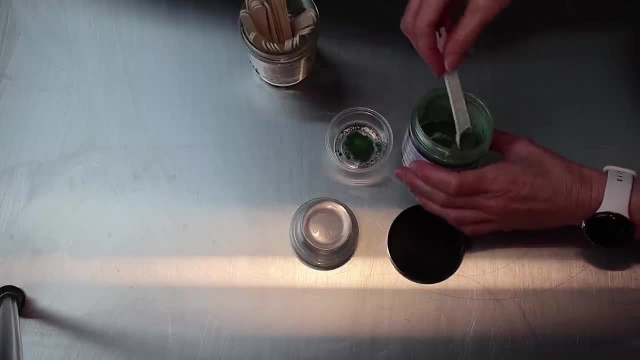 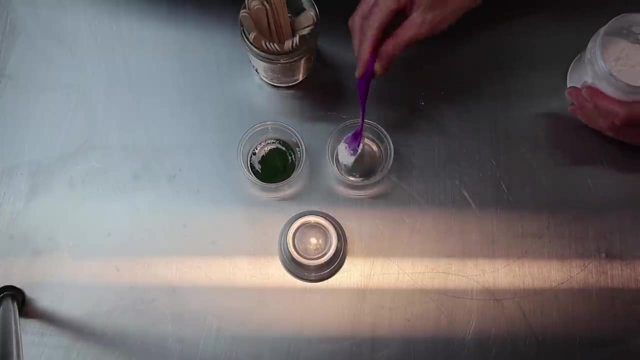 that I mix these in And right now I'm out of the containers that I like to use, but these will do With anything. you kind of learn as you go, The more you do it. you kind of find a routine that works for you. 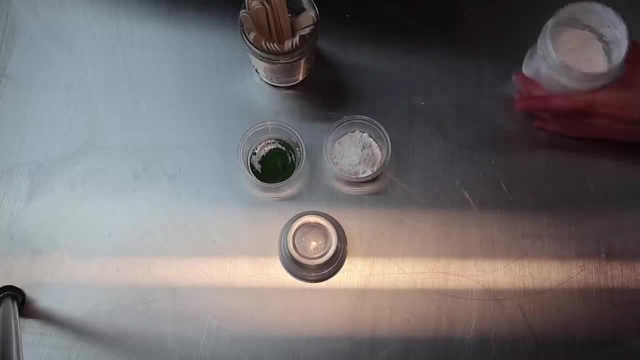 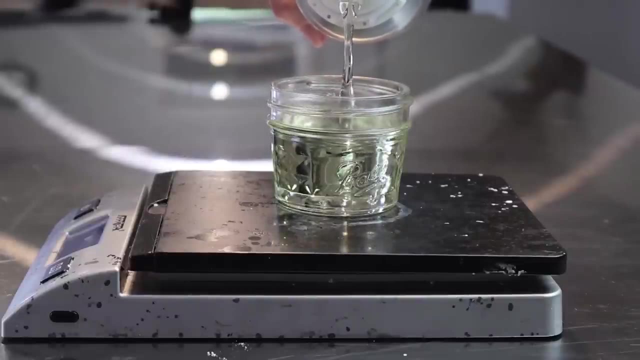 I've even learned that during the summer, I can wait to do this prep work until I have my lye and water mixed together. Since it's warmer on the outside, my lye water is going to cool down slower, allowing me some time. 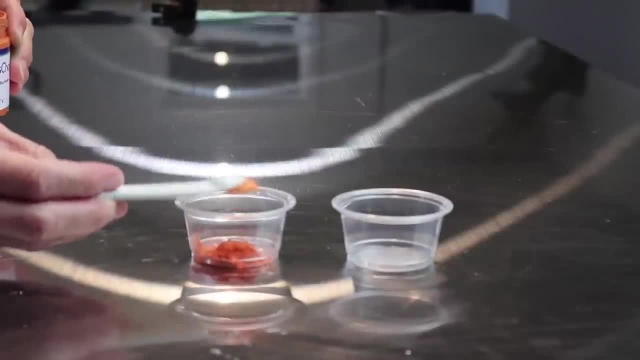 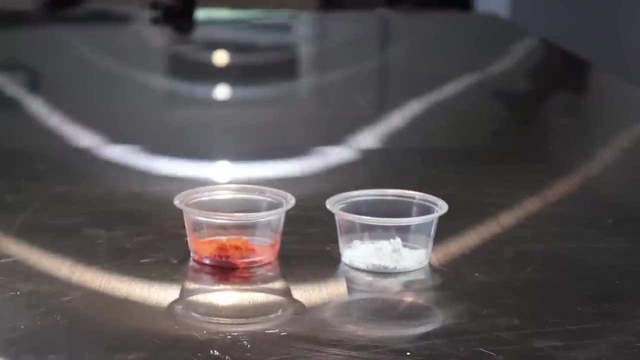 to do this. I always try to fill all of my minutes up with doing something valuable, and I don't want to just sit around and wait for my lye water to cool down, So it's nice to be doing something as that is happening. 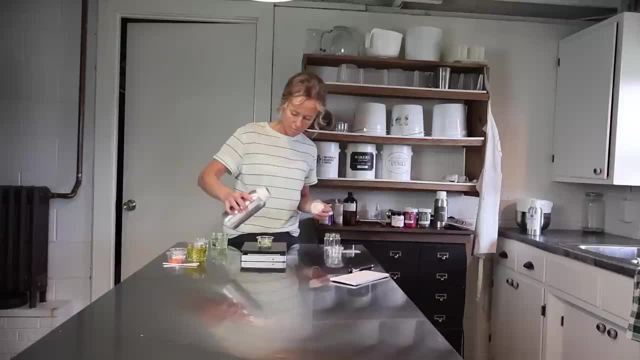 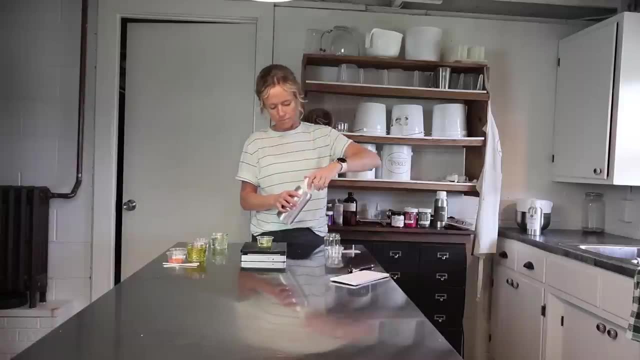 I was so disappointed in myself Here. I wanted to make this relaxing video with some sound effects. I'm going to include it as I'm working and I accidentally left my mic plugged in into my camera, so that would mean there's no sound in a lot of the clips, But hopefully it's. 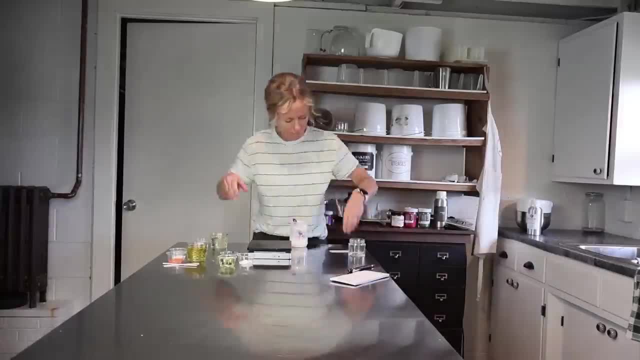 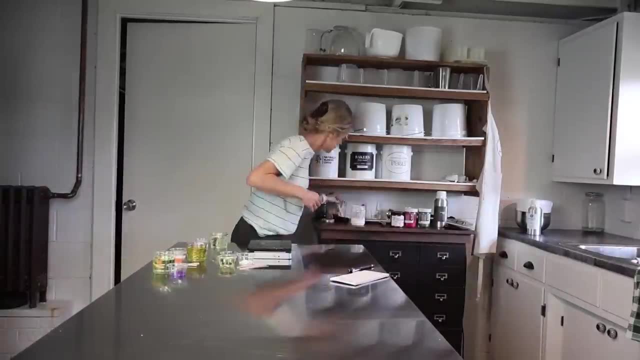 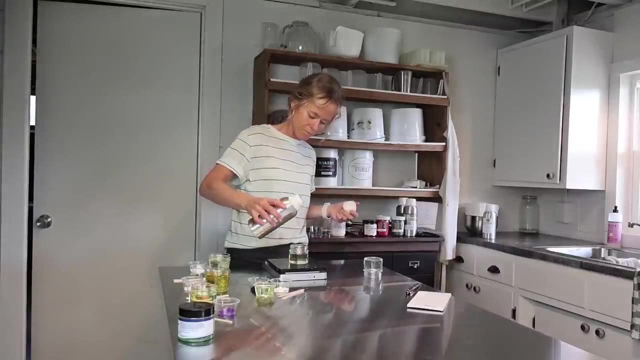 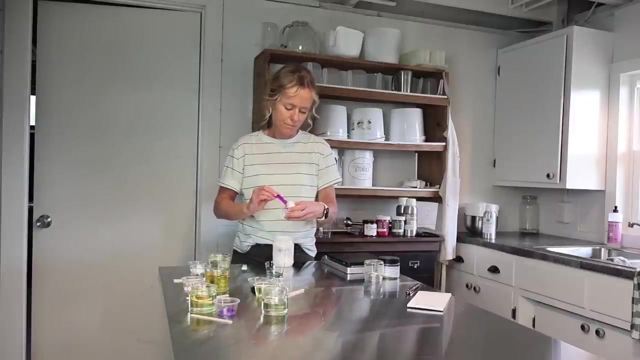 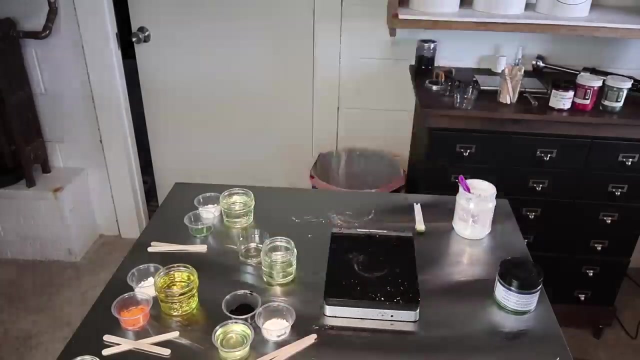 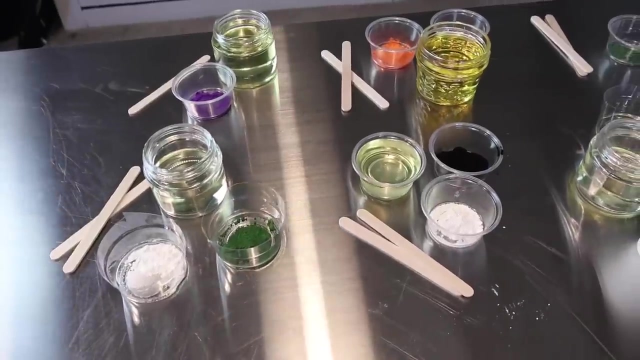 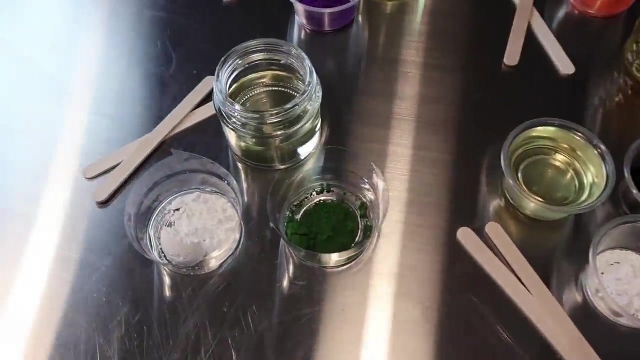 still relaxing for you guys with the music. Here's all of my prep work. as far as the scents and mica powders go, Probably looks kind of confusing, but I think I know where I'm going with it. Hopefully Here is going to be my new swirl, that I'm going to try And it's supposed to look. 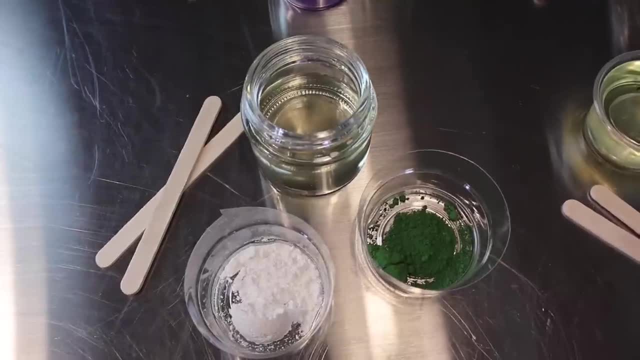 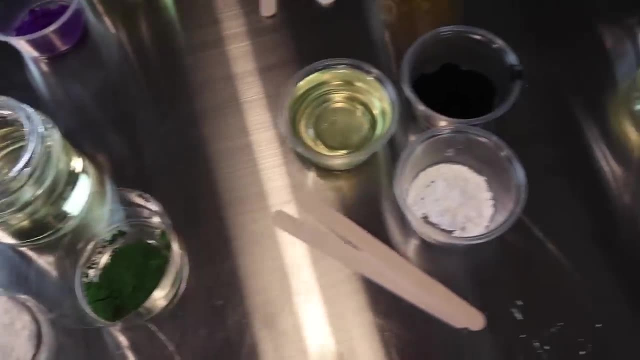 like grass by the time I'm finished, like the swirl or the streaks in the soap, rather, and the scent is aspen grass smells so good. and then over here is another new one, that on the fly here I decided to try this. this one is: 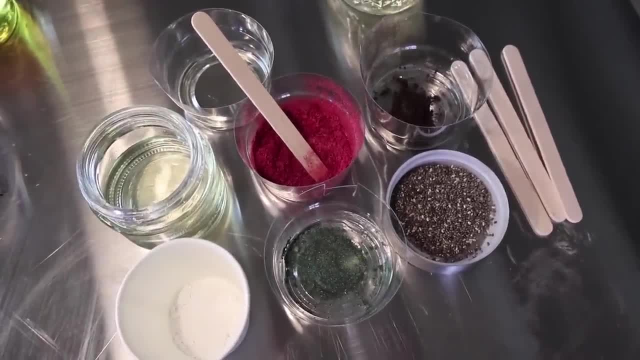 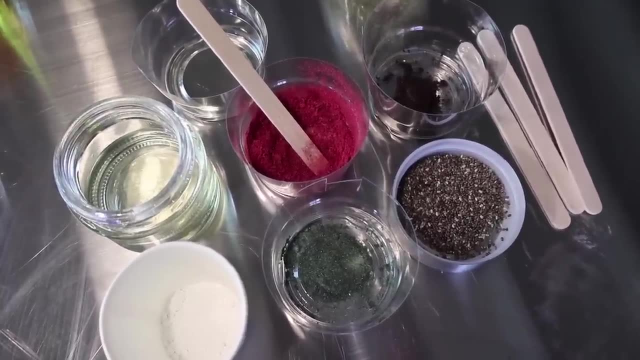 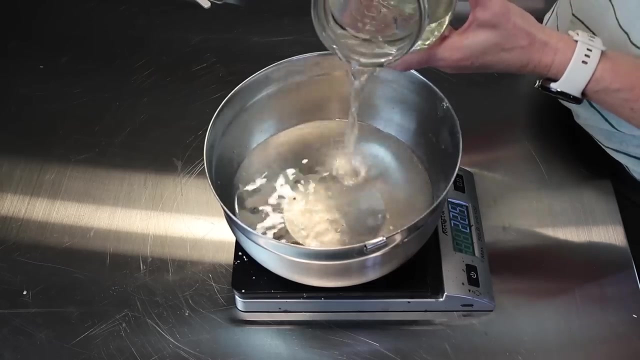 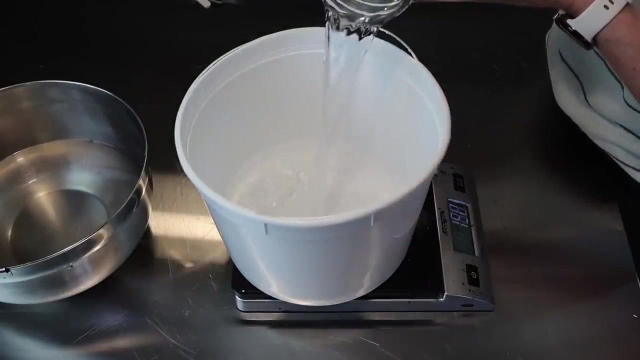 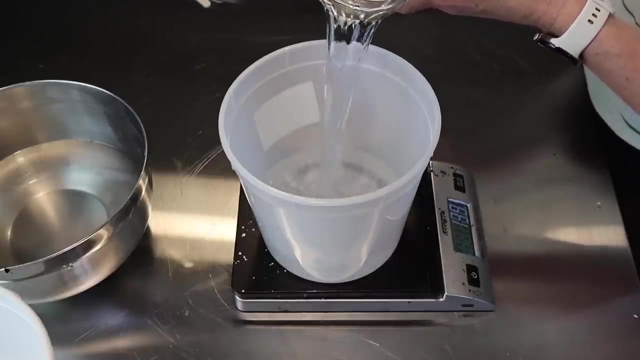 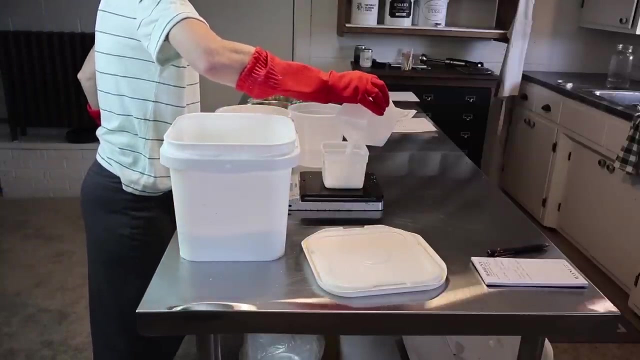 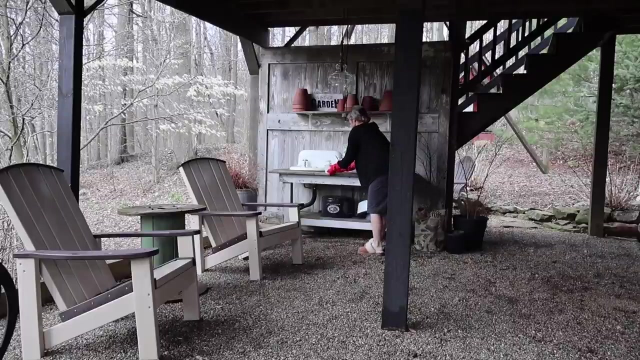 probably going to be the biggest challenge, as you can see lots of different ingredients. but to make a long story short, I want it to look like chocolate covered strawberries by the time I'm finished. so we'll see. you always make sure to wear proper gear when mixing lye and water together, of course. 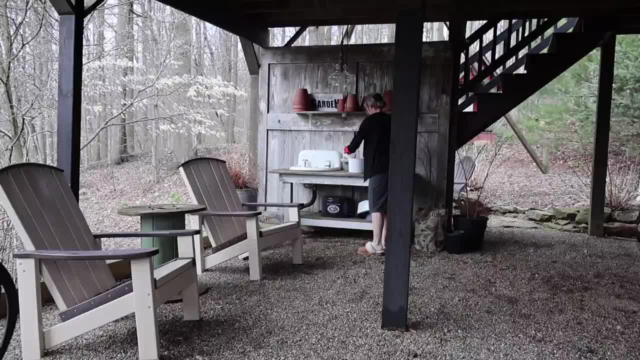 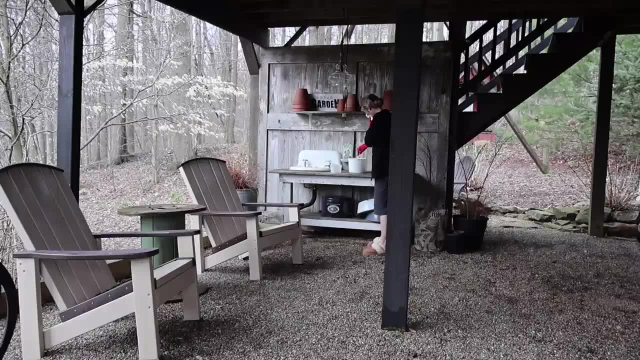 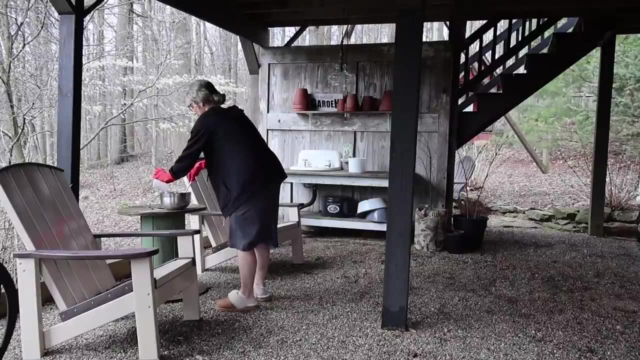 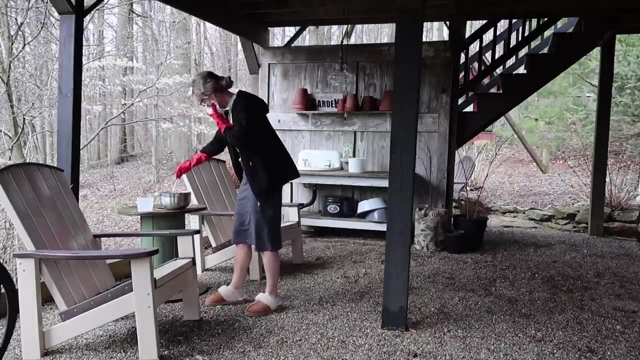 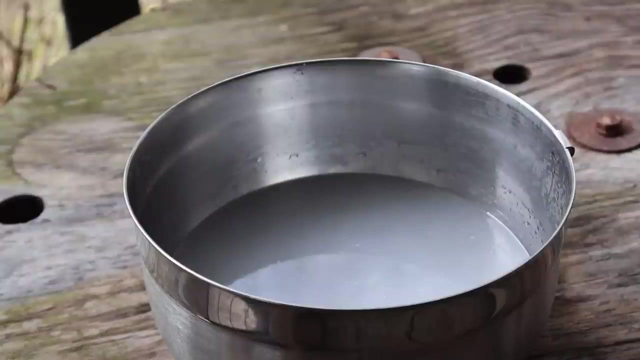 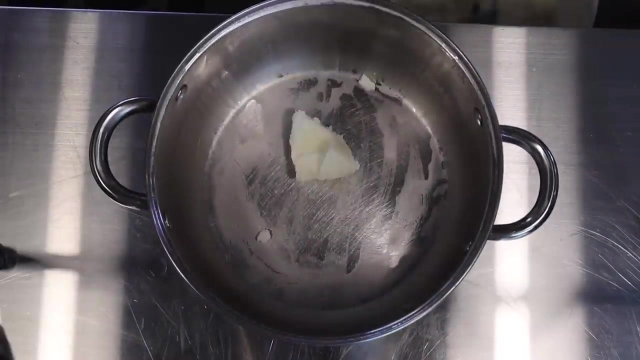 and I always try to watch- you know which way- like the steam goes, and I try to stand away from it, and I also have a mask that I hold over my mouth and nose to breathe through, so you know everything that you want to see. my favorite thing about the street is that there's- you know there's- a lot of. 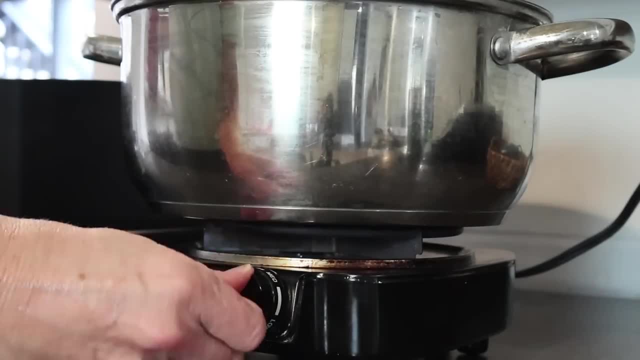 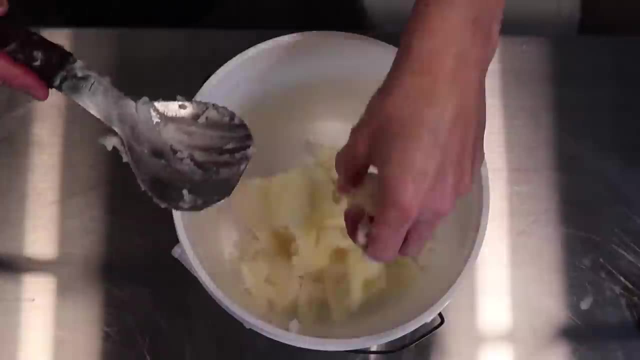 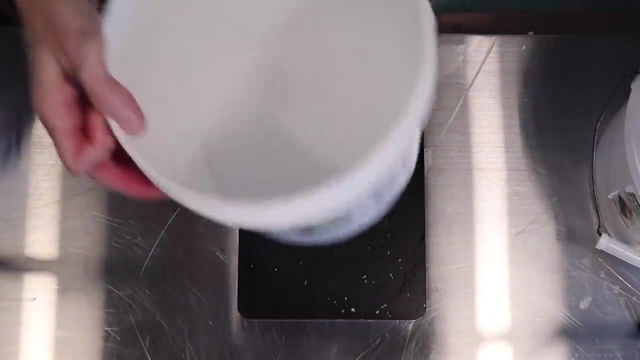 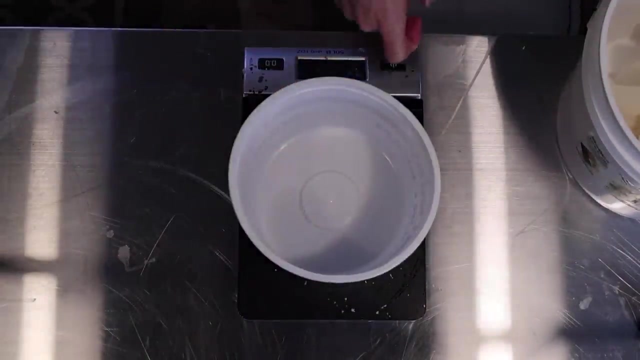 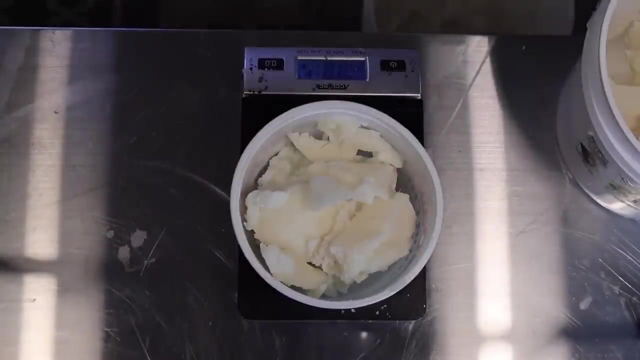 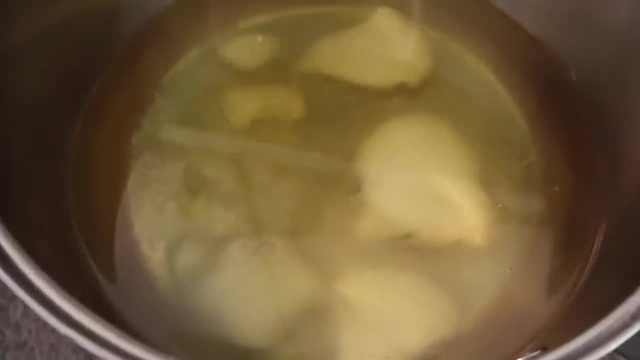 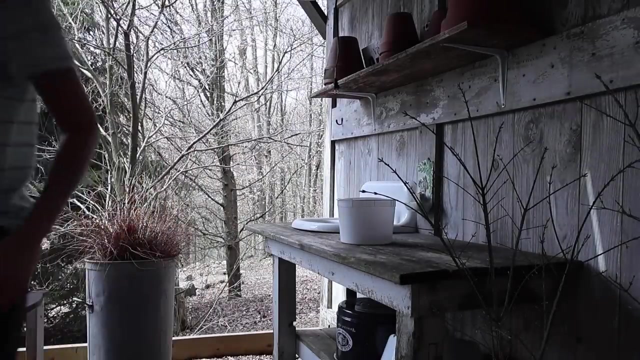 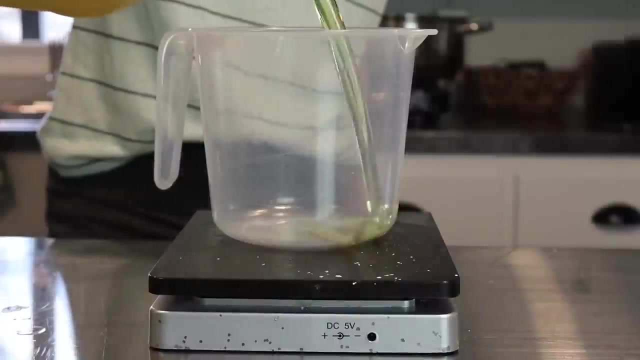 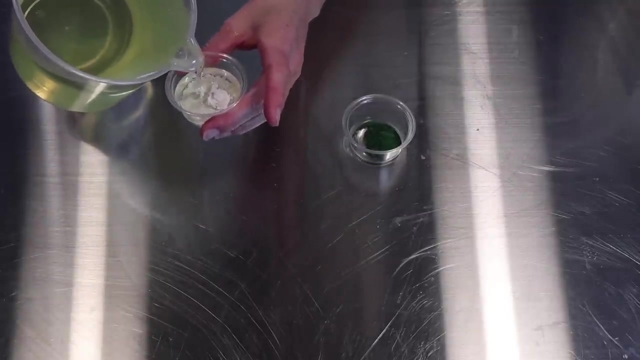 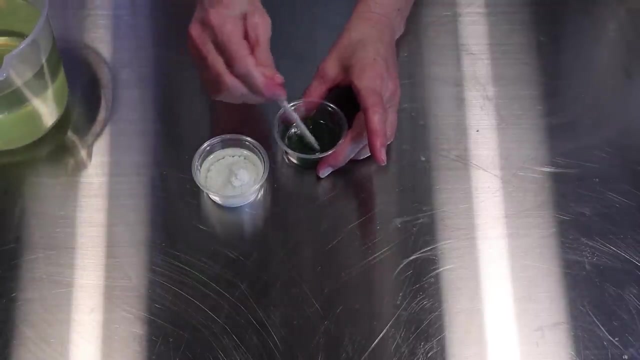 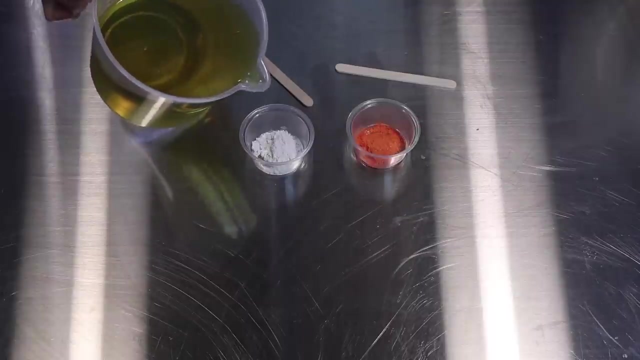 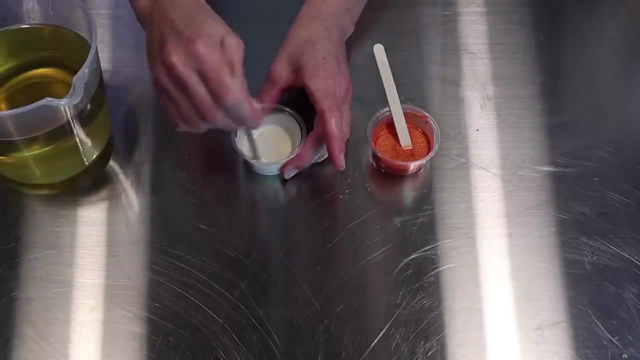 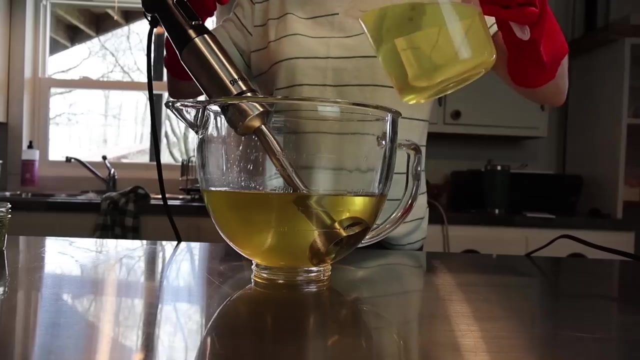 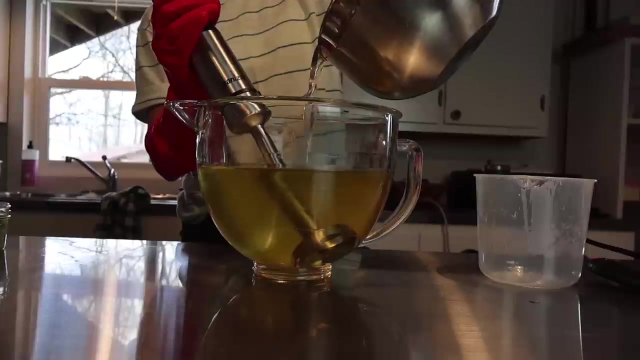 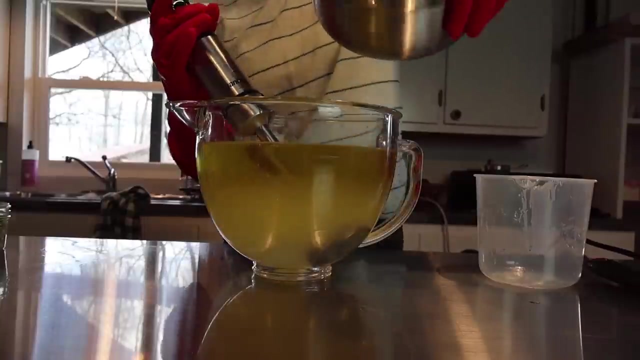 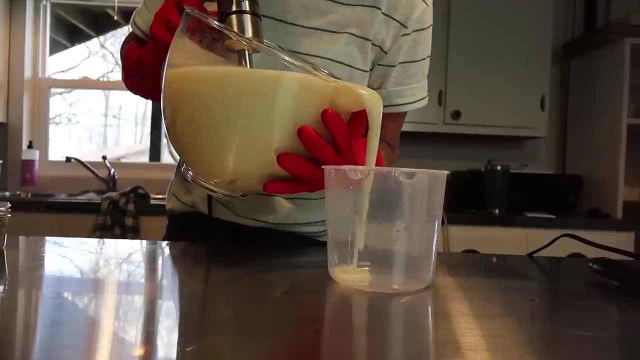 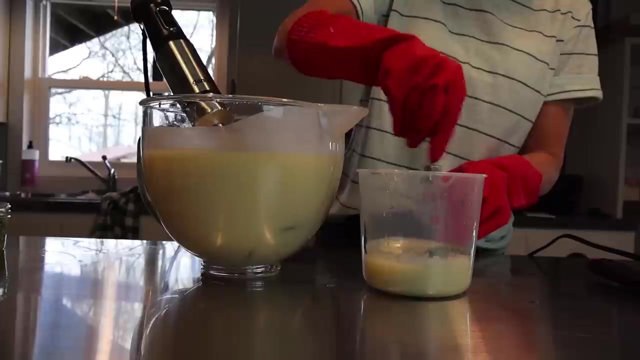 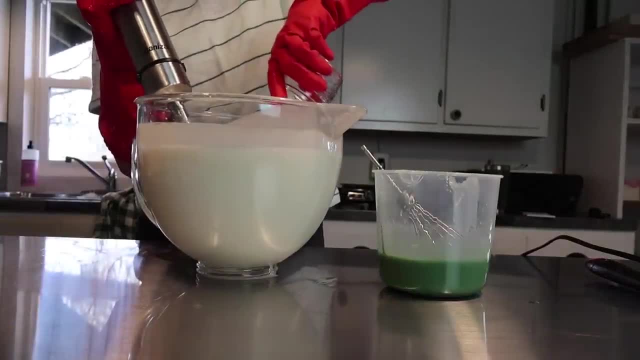 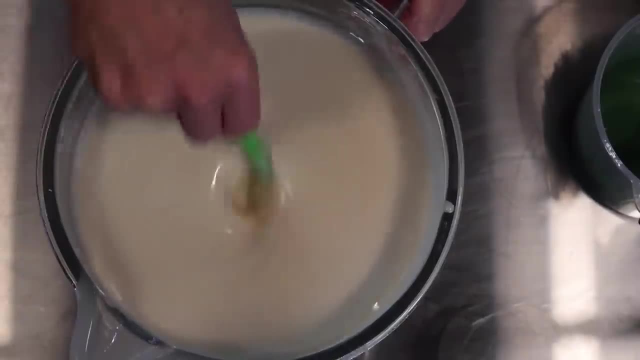 And I want it to reach like a medium trace is often what I go by And if you're into soap making you know what I'm talking about. But your trace is basically you know how thick it is And often I'll test it and kind of drizzle some of the batter you know over the top. 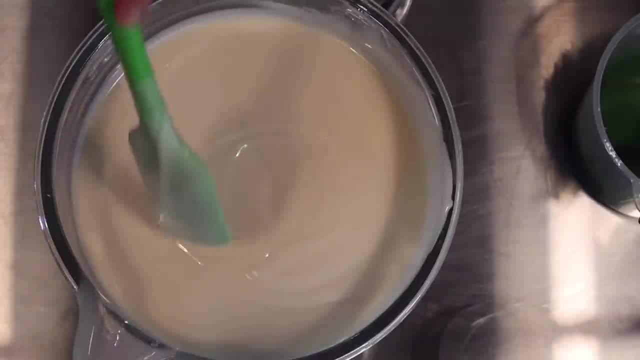 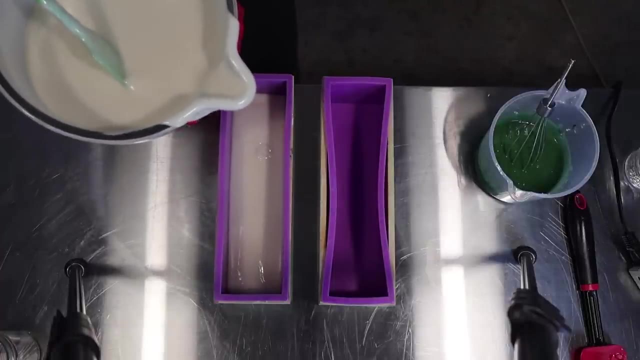 If I can still see some of the marks, it's about right to pour. A normal batch of soap that I make fills two loaves, And these are molds that I get off of Amazon. They're just small. They make a nice nine bars plus a little bit of extra. 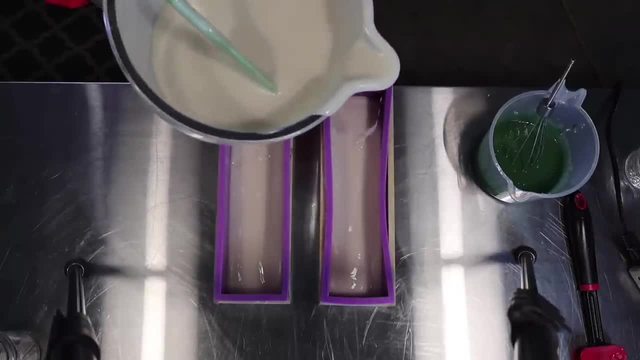 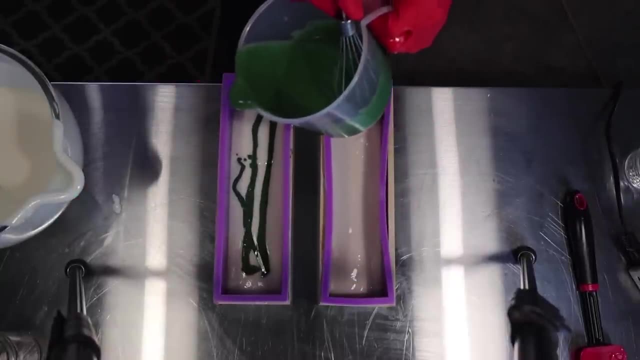 And I'll link them down below in the description box, along with any other tools that I use here. I do have a recipe for just a single loaf And I'll use that one if I make any samples or something new For the first time. 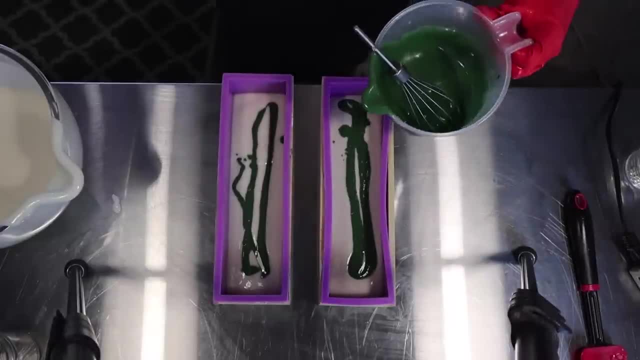 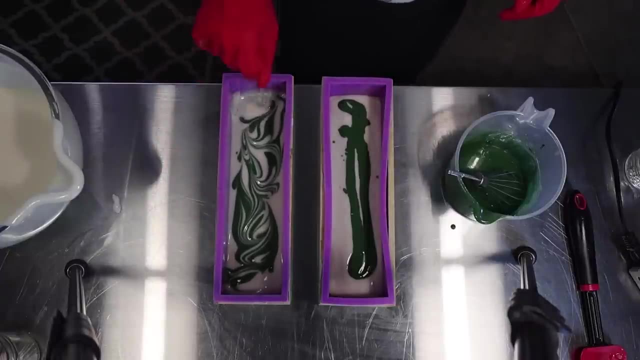 And I also have a third recipe that I use to fill a round soap loaf And I got the mold from Brambleberry And I'll try to link that down below, also in the description box. I just recently started making round soaps. 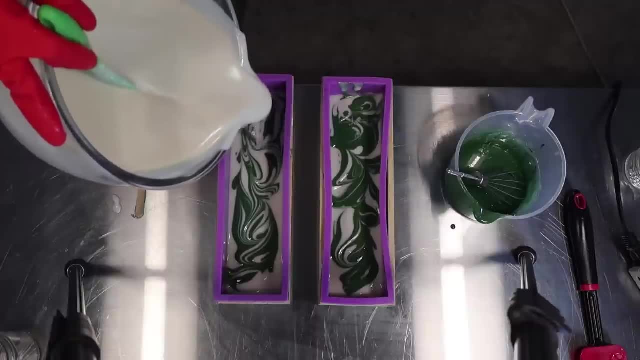 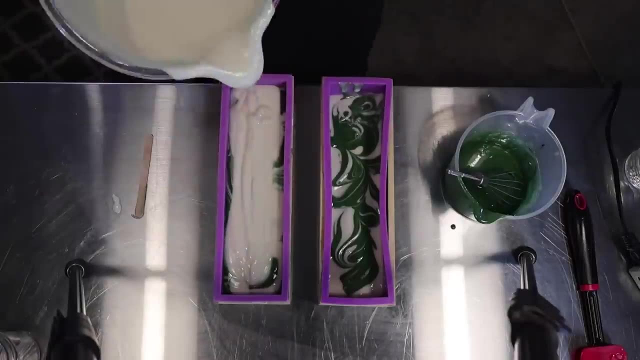 And I definitely should invest in a few more molds. It will be more time efficient to do that, But for now I'm having a lot of fun with dabbling in round soap. I started doing somewhat of a different swirl than I used to. 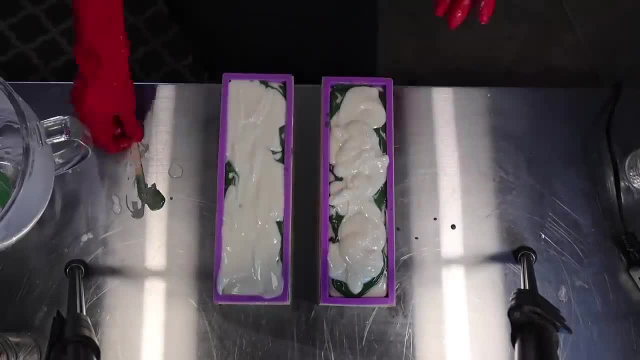 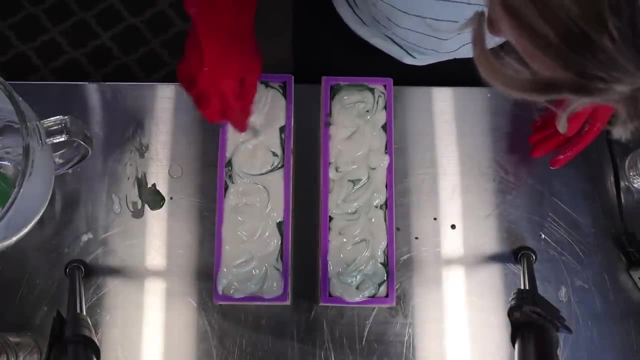 At one point I would just mix my green batter into the white as it's still in the bowl like a drop swirl, And then as I poured it would kind of mix together in the mold And I found that often I'd get almost a light green soap versus a perfectly white and green soap. 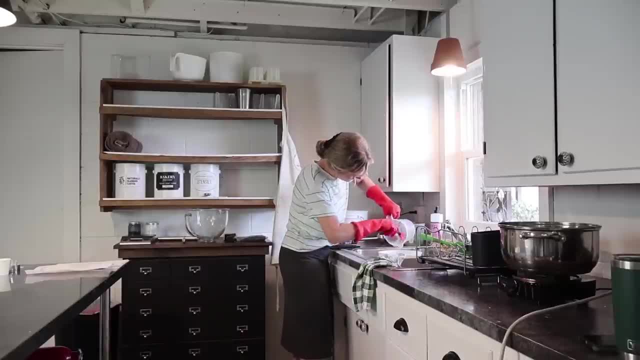 So this way what I'm doing here definitely helps with keeping the colors kind of separated. So my normal space to actually mix the soap is over here by the sink. So I think my next batches I'll be doing that. I've found, you know, time. 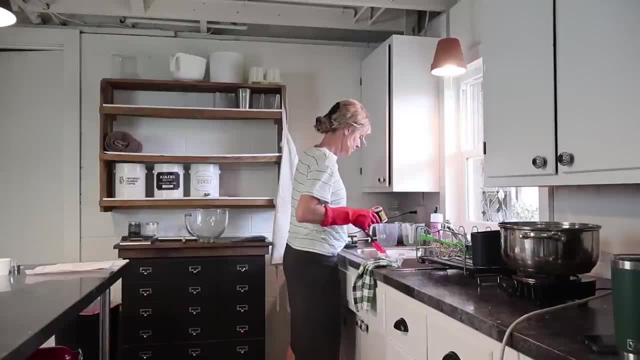 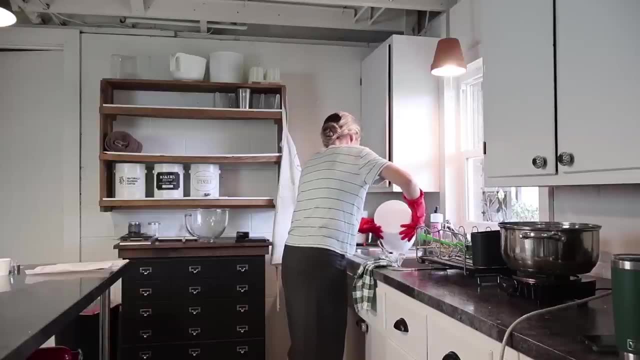 Time is everything when you're making soap like my lye, water is cooling on the outside. I need to keep at it and it's just easier for me to work in my space that I'm used to. I did that first batch on my island table so that you could see- you know what I'm doing through a glass bowl. 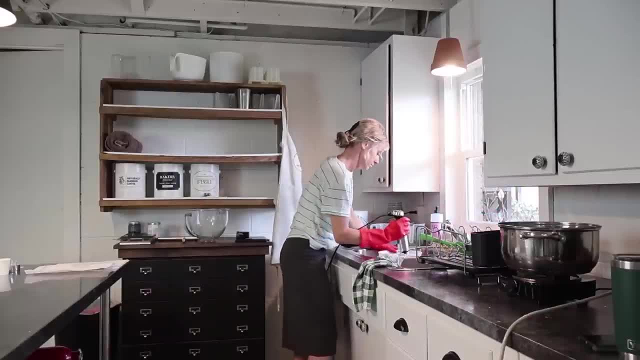 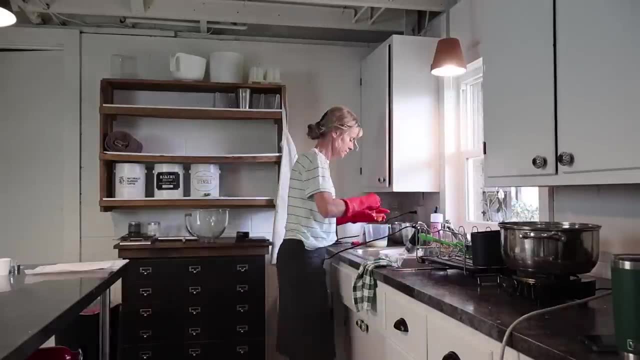 But it's basically. all of them are the same, you know, just being mixed together. The second batch I'm doing here is Citrus Grove. It's one of my favorites too. It's MB's favorite. She loves this one. I did mix just a little bit of chamomile. 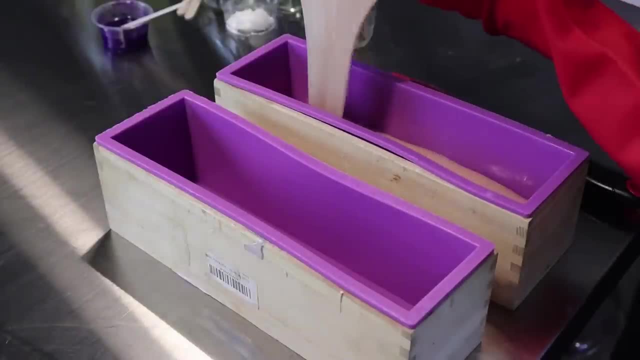 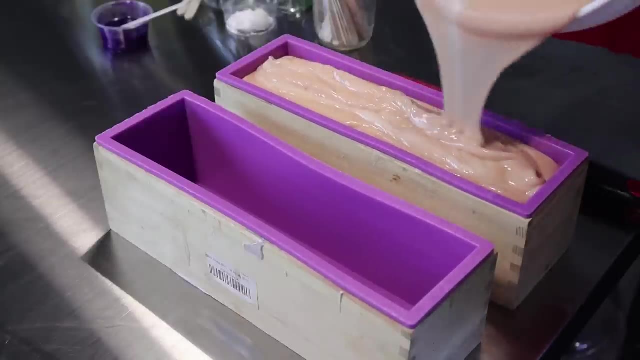 With this. so it's kind of an orangey chamomile scent. And for the swirl I'm actually doing the old way as far as I'm pouring my white mixture into the bowl that is filled with the orange batter, And I thought my camera was rolling when I did this, but it wasn't, so I kind of missed. 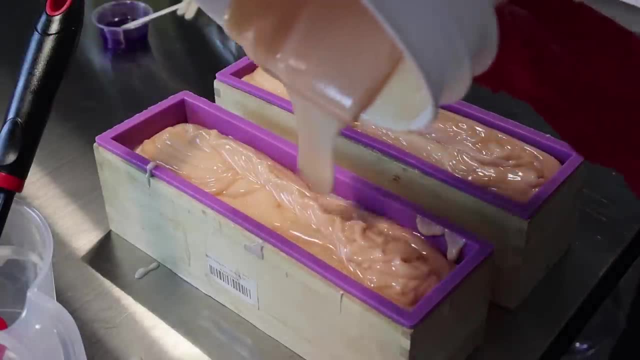 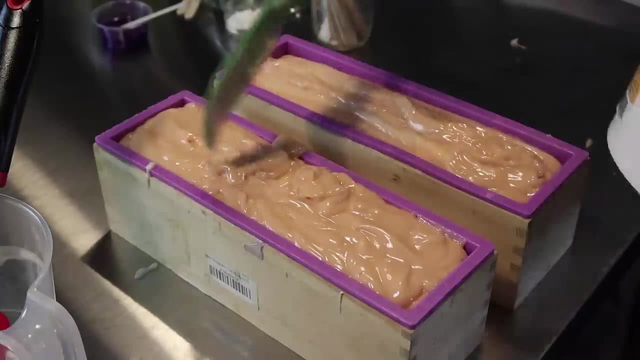 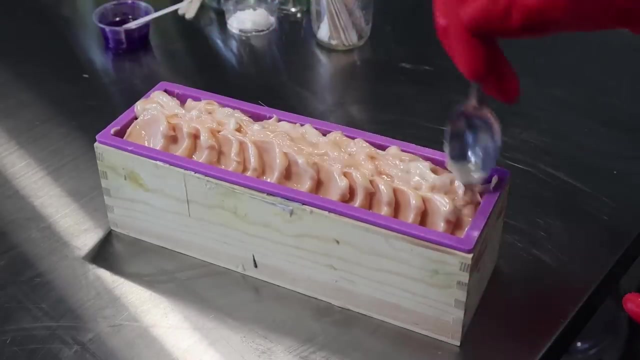 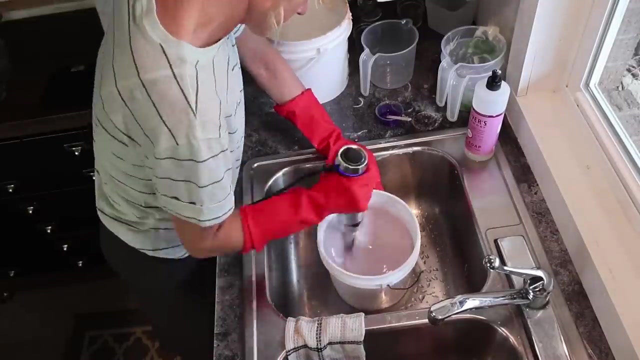 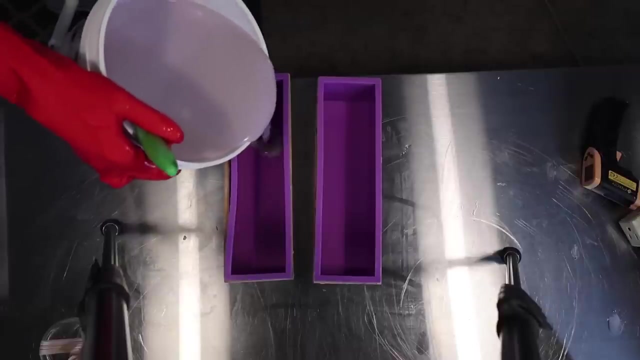 filming that, But that's what I did here. This one is lilac and this is our same old lilac scent that we've had ever since I started making soap- Also one of my favorites and, in case you can't tell, I'm really into floral scents. 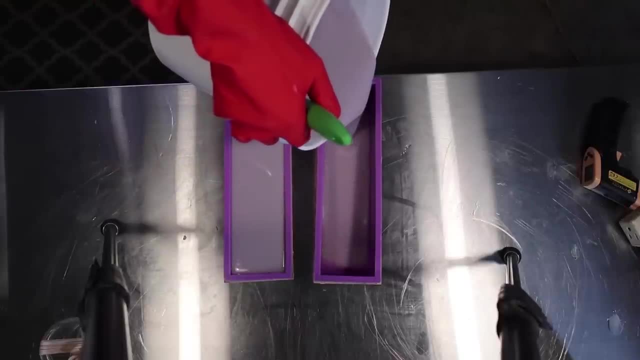 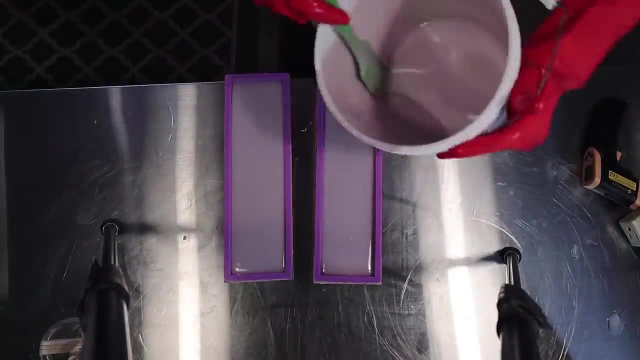 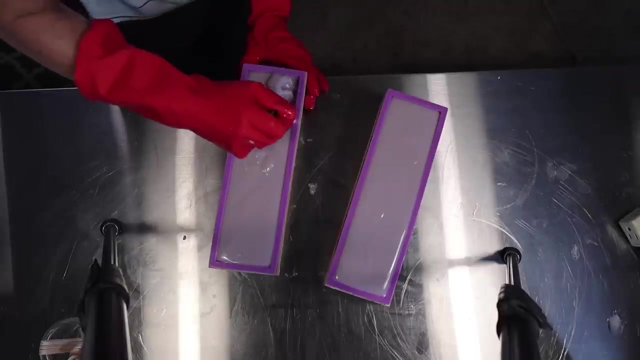 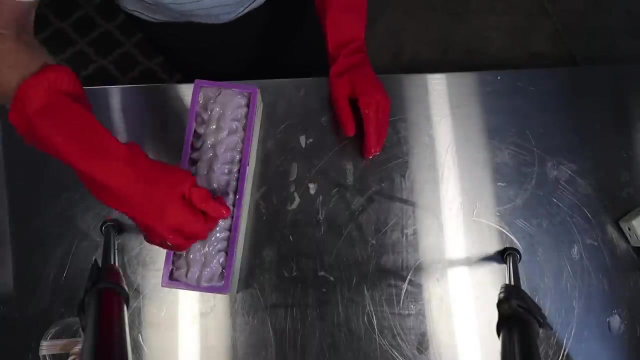 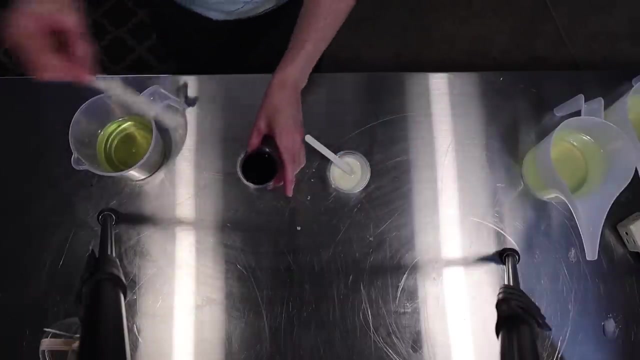 And this color is just lovely. It just fits exactly how the soap smells. It's just a pretty soft lilac color. For my round soap today I'm going to do the Wild Blackberry And this smells wonderful, but I kind of forgot. it does accelerate and that means some of 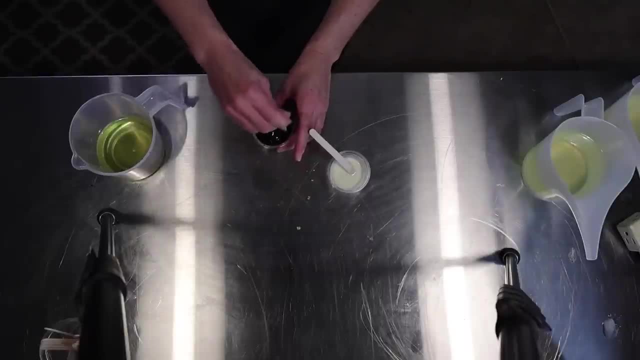 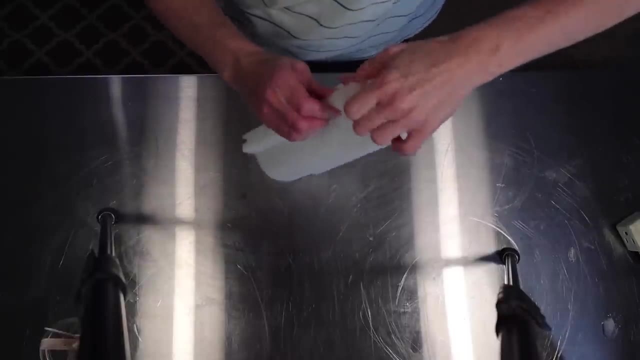 your essential or fragrance oils, The oils that you add into your batter will make it accelerate or get thickened too quickly And I have to work quick here. but I see I'm not getting my white mixed in with the black like I want to. 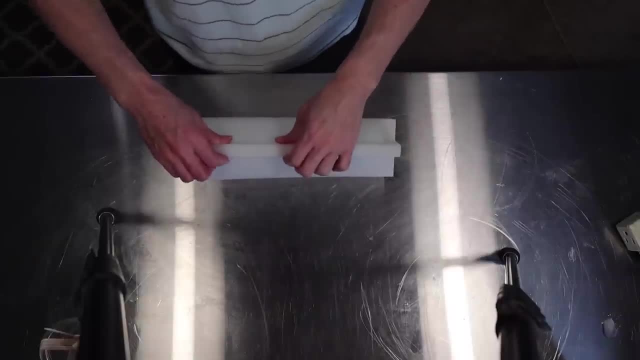 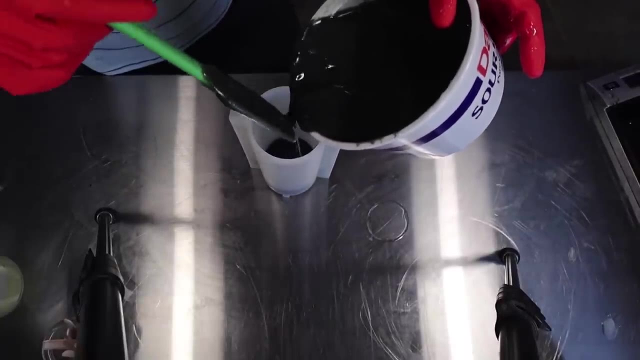 I should have just hand mixed it. That also helps if you run into that. Not use your immersion blender, just hand mix with a spatula. And I haven't mixed this one recently and I kind of forgot that. that oil, the blackberry. 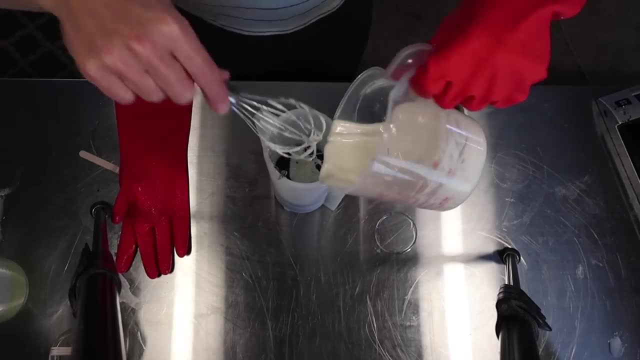 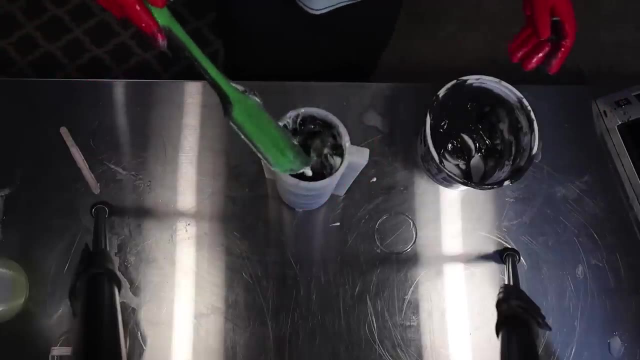 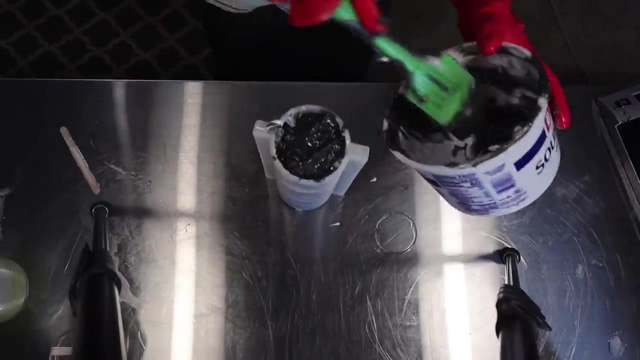 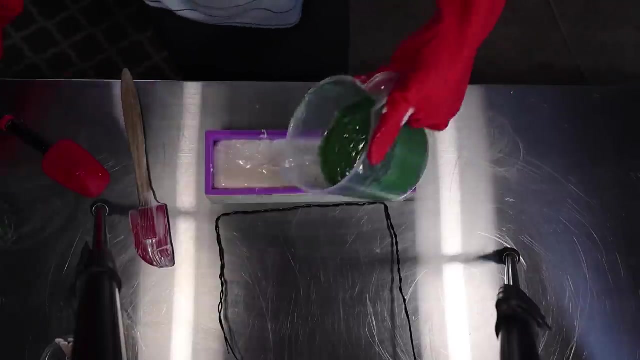 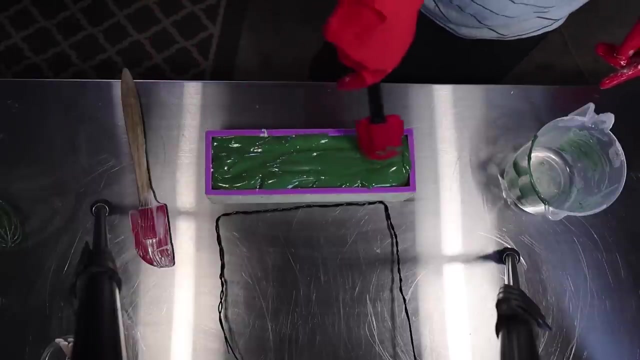 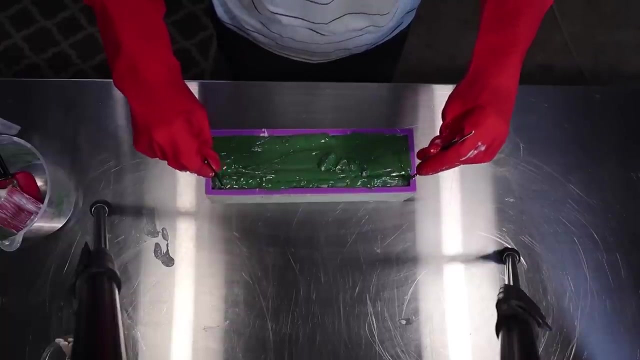 oil kind of does this, but it'll still smell great and work the same Might just not look quite as pretty, So the swirling method I plan to use here for this grass soap is a- It's called a hanger swirl, and it's where I put this piece of wire that I twisted together. 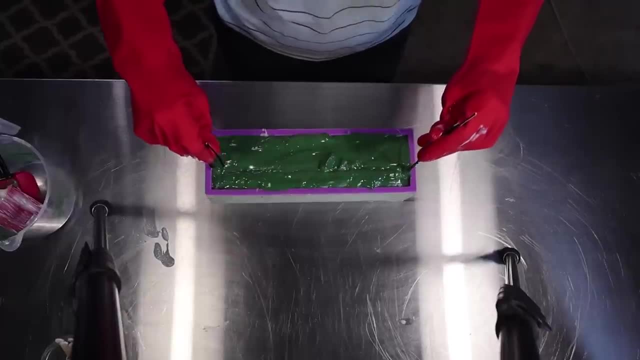 just to thicken it a bit, Kind of put that in the mold and try to push some of my green down into the white Again, trying to make it look like blades of grass. I have no idea how this is going to look, but I do know it's going to smell great because 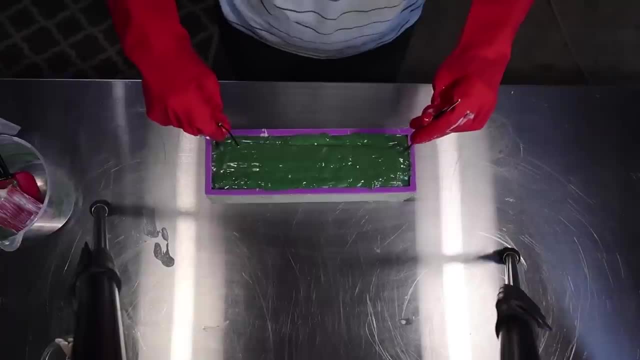 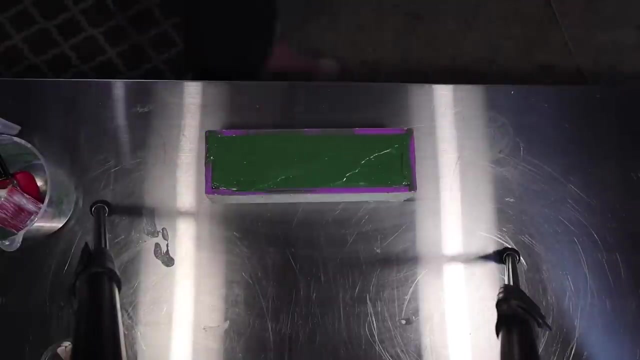 I love what I'm smelling, So I guess it doesn't always have to look pretty as long as it functions, but definitely a plus though, if it turns out. So the final one here is again supposed to look like chocolate-covered strawberries. 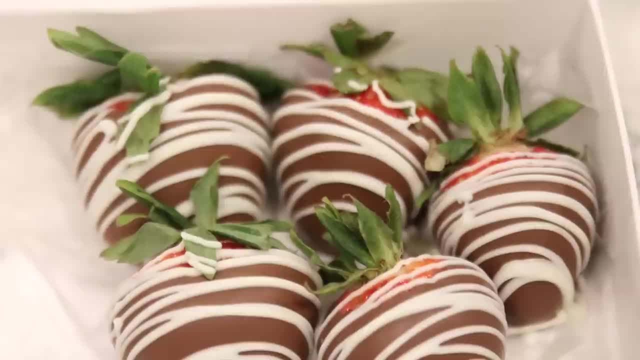 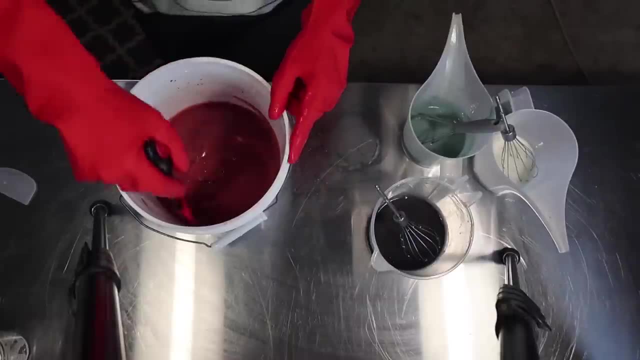 I took a picture recently- I think over Valentine's Day- of some and I just love the color combination. I thought I'm going to try to make soap to kind of look like this. The main part of the soap will, of course, be made to look like strawberries, and I'm using 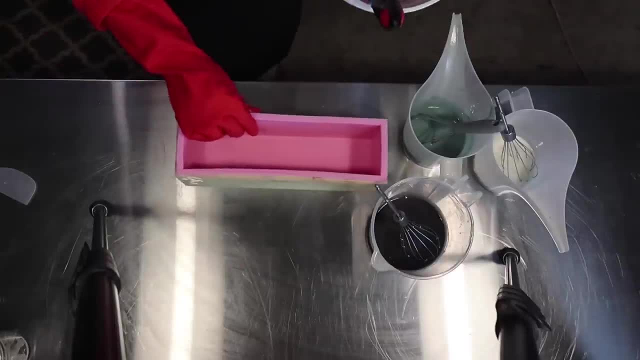 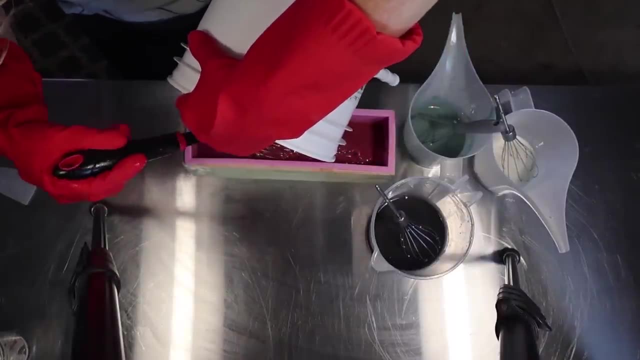 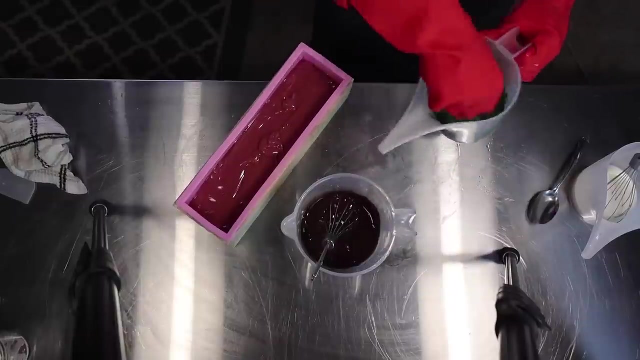 chia seeds. I'm mixing that in here to have that strawberry seeded. look Okay. So I'm going to mix that in here. The green, of course, will be for the leaves, and then I have a brown for the chocolate and I'm going to drizzle it with the white. 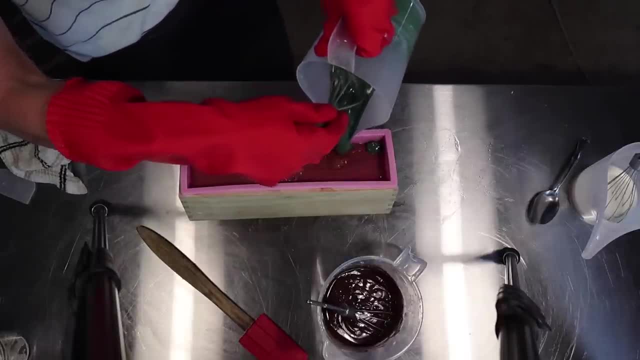 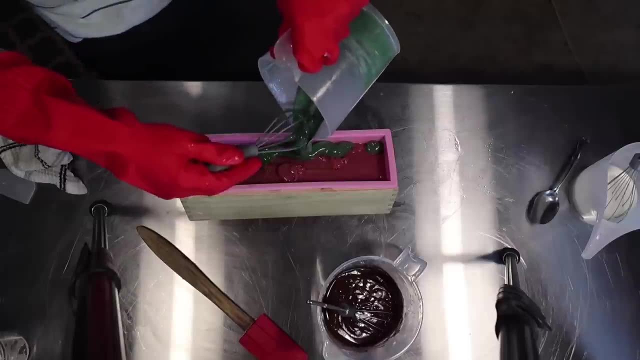 And as I'm mixing here, I already see I don't have my amounts proportioned correctly. Like I have too much green, I think, and the green should be a little bit lighter. It's not quite the shade that I was thinking of. 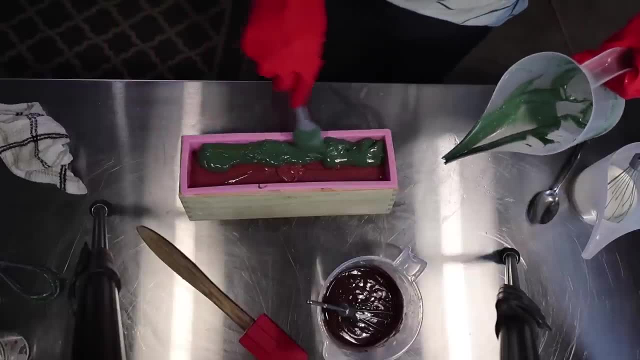 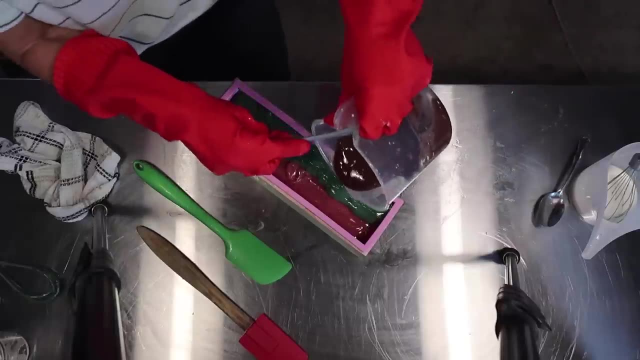 And then I think I have too much chocolate and white too. So definitely, if I decide to do this again, if it even turns out, I'll probably do more strawberry and just a lot less of all the toppings. I actually used a cocoa fragrance oil to scent my chocolate part with and all of the other. 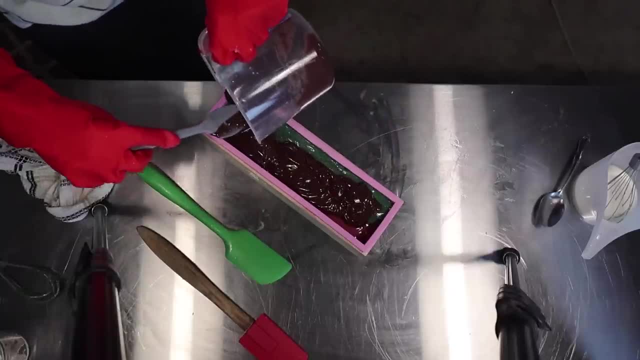 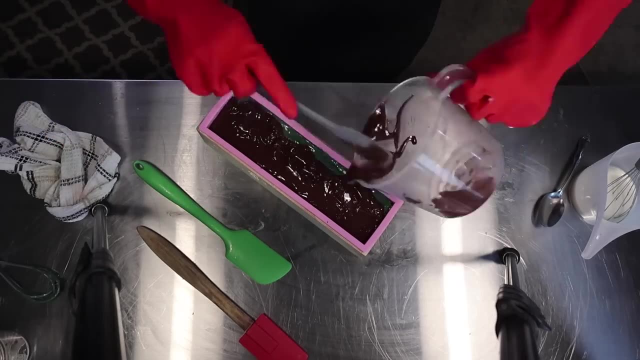 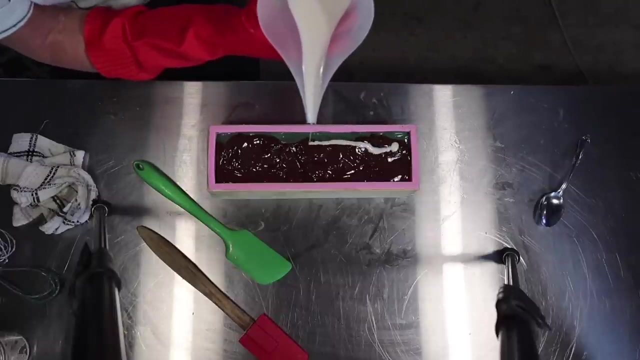 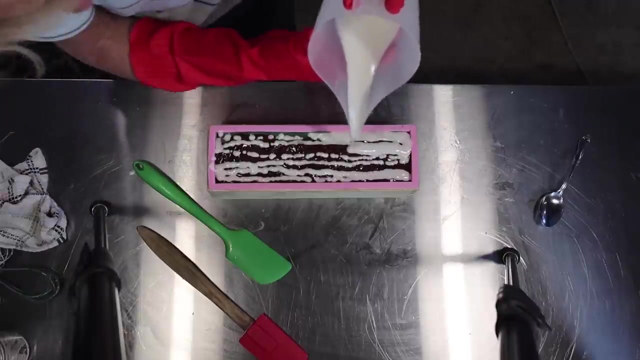 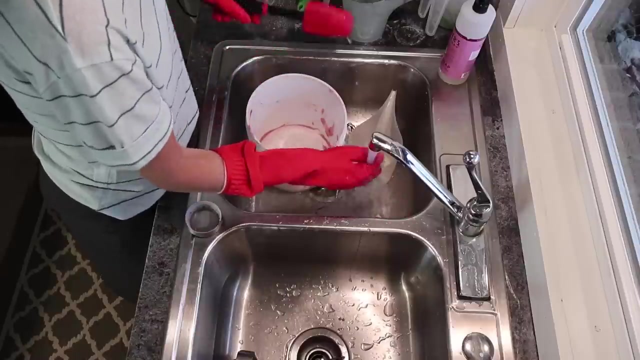 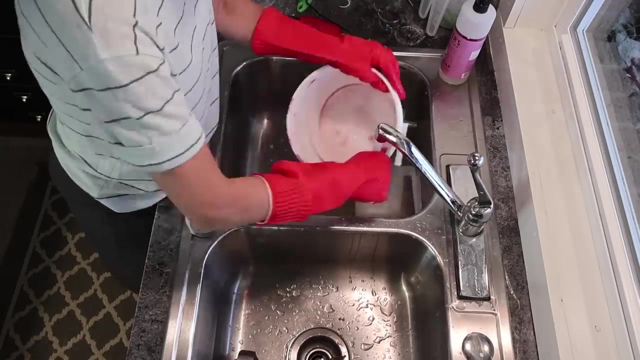 colors are scented with the strawberry And I got to say it smells exactly like chocolate-covered strawberries. right now It smells so good. Of course there's going to be some dishes to wash with soap making. I always pre-rinse everything before I actually wash it. 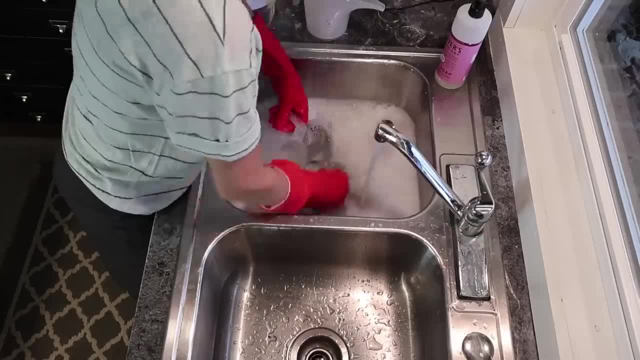 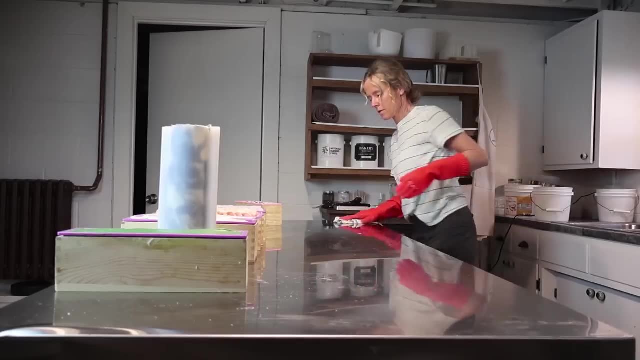 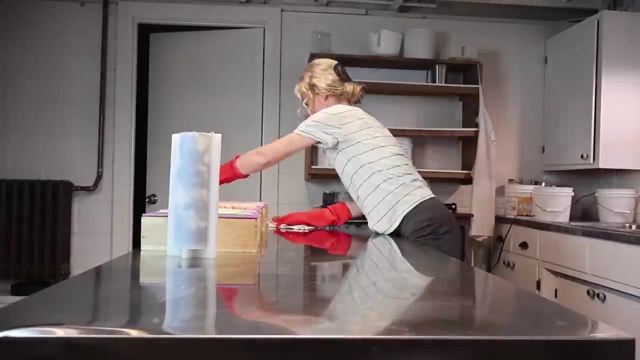 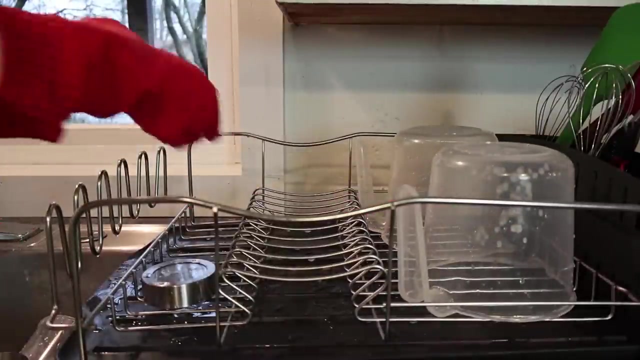 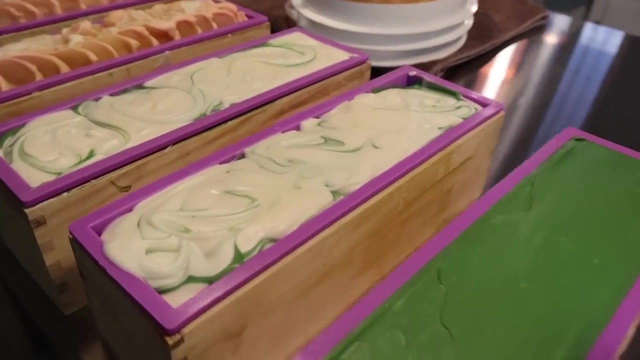 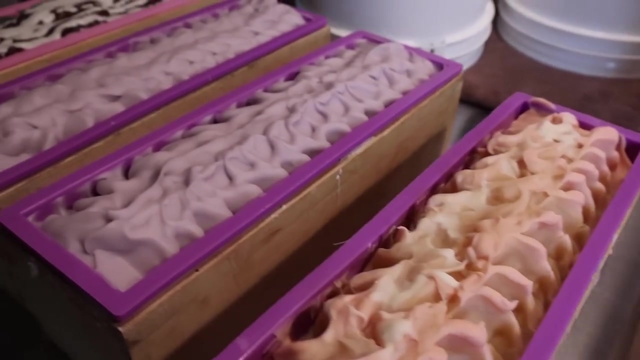 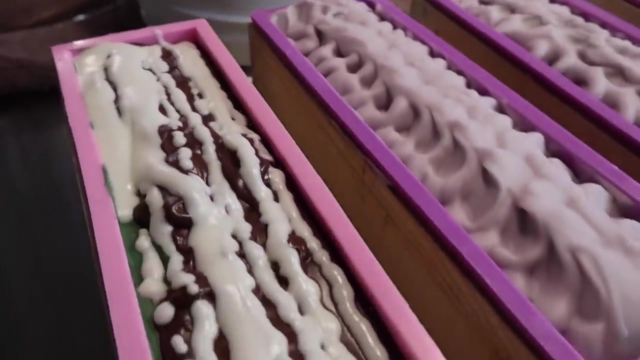 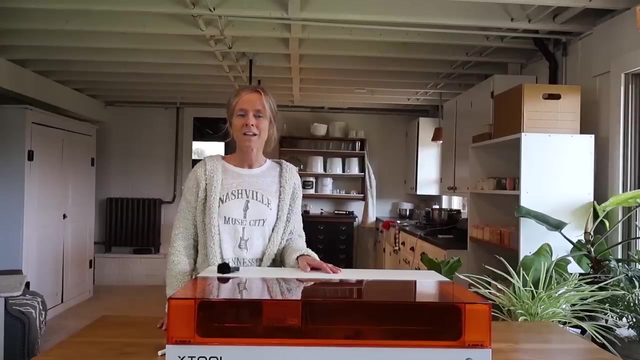 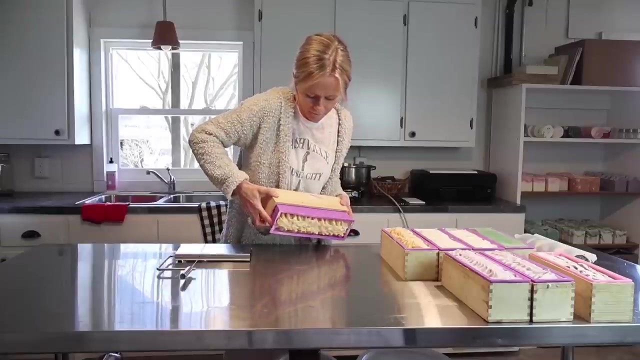 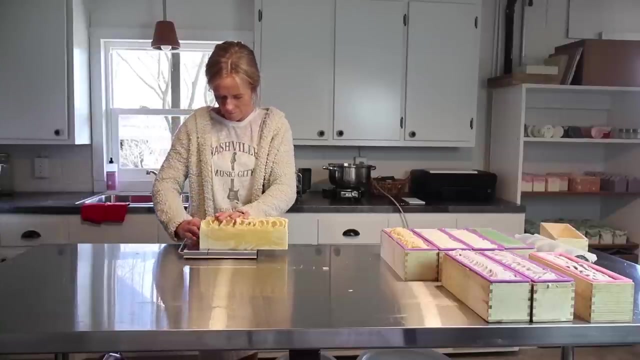 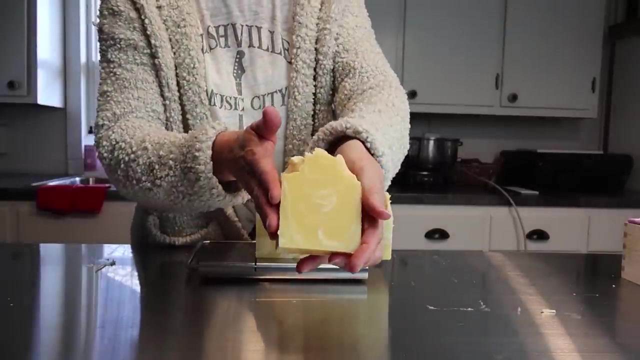 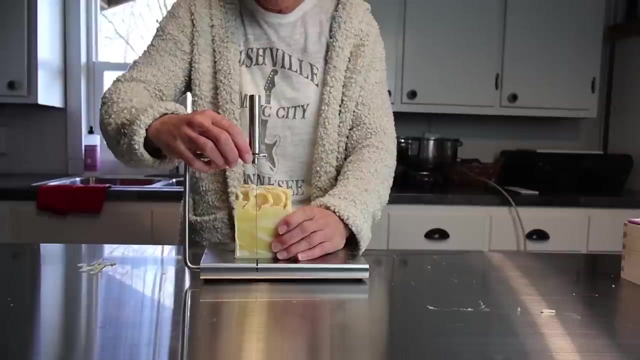 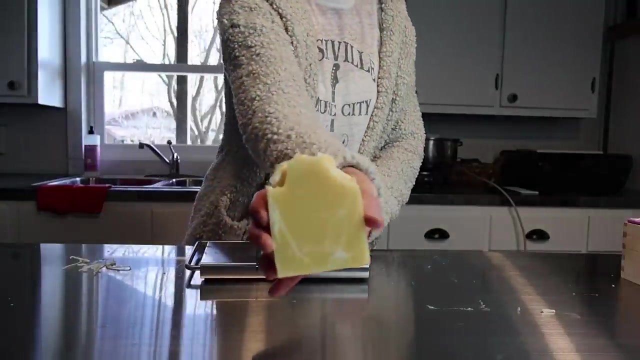 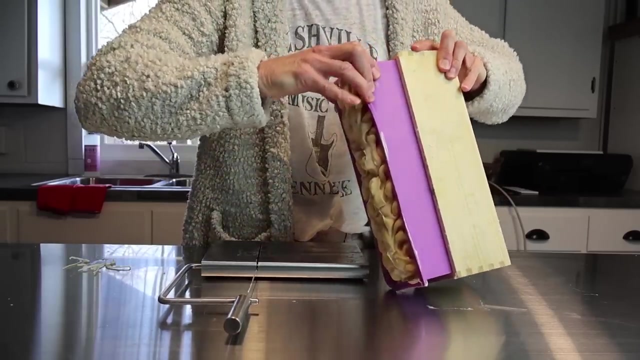 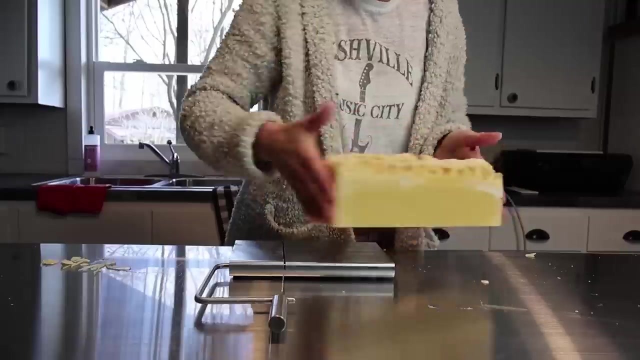 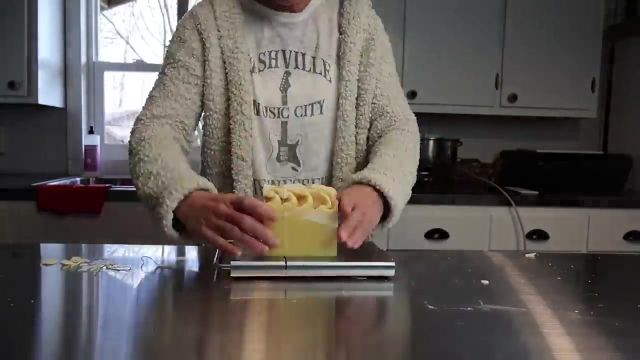 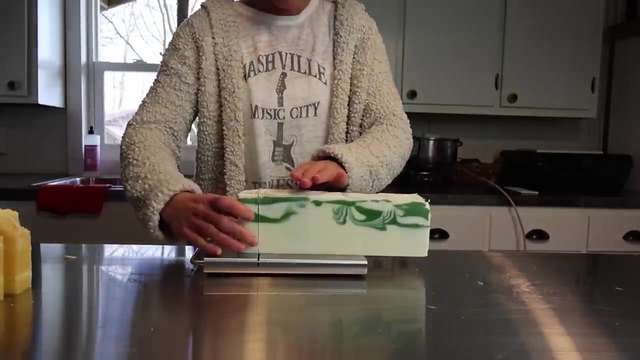 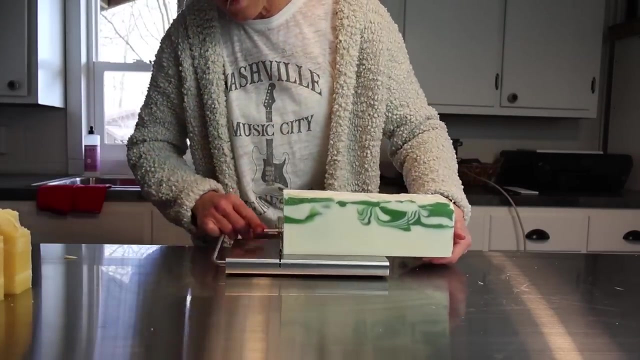 Okay, Okay, Let's go. now. we have the fun part of cutting and labeling the soap. it's always so satisfying. I can't wait to see what those two new samples look like on the inside. so let's find out. you, you, you, you, you. 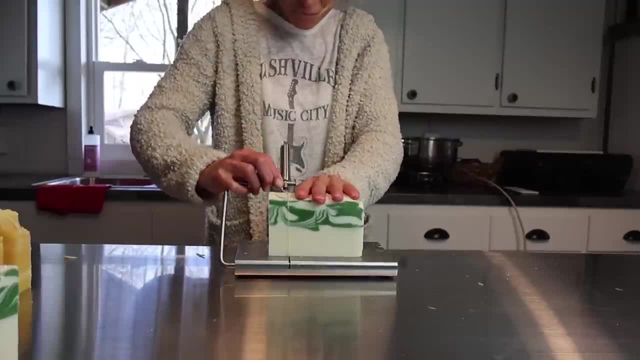 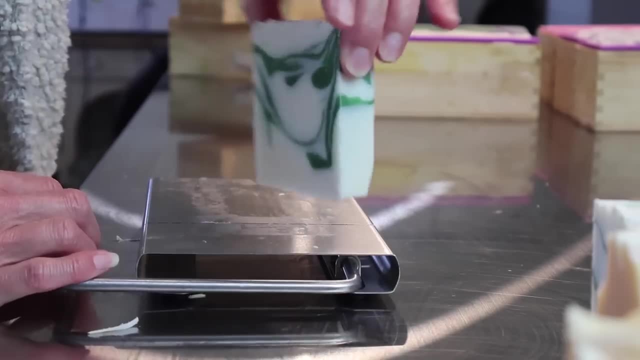 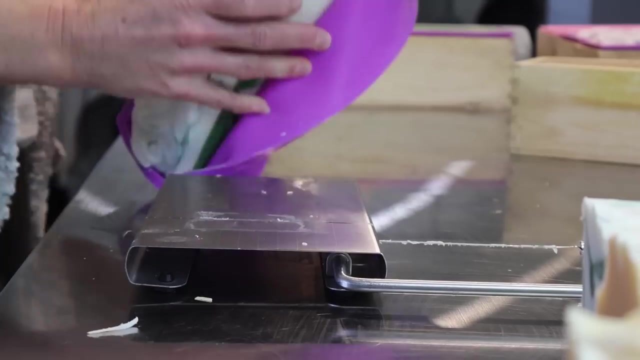 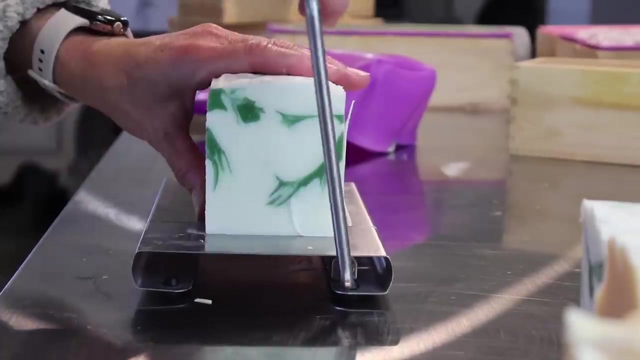 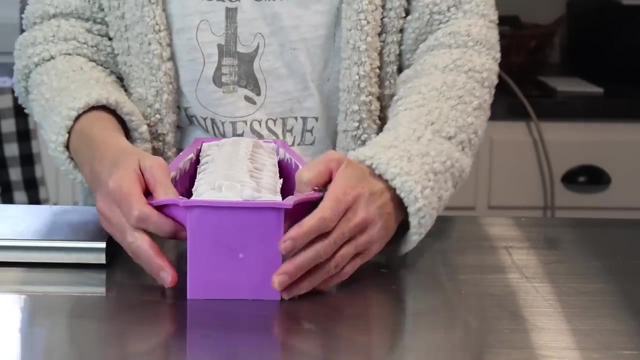 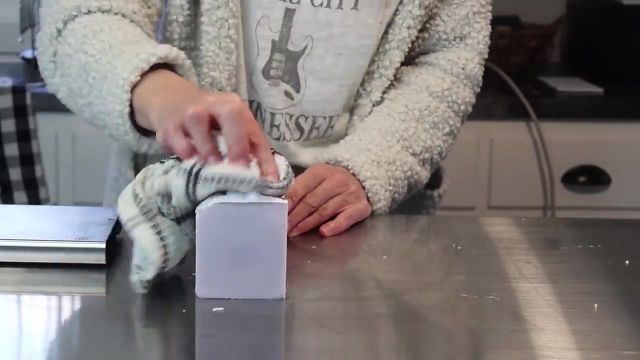 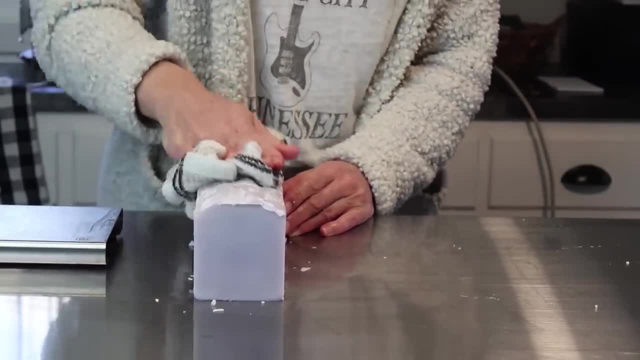 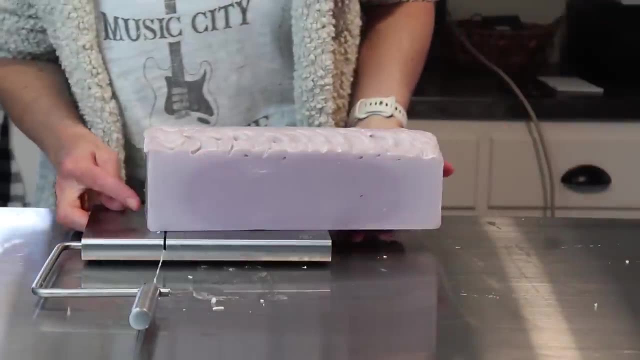 mysteries, I guess, is why some loaves get it and others don't. I've done a lot of research, tried to, you know, tweak things here and there and I just haven't really figured out a way to completely avoid it. but it's. there's worse things that could happen with your soap. I mean, it's usually. 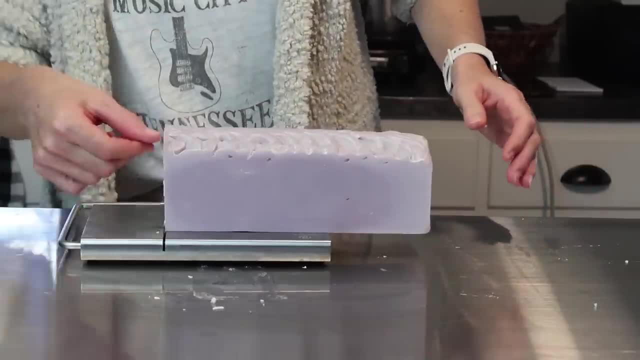 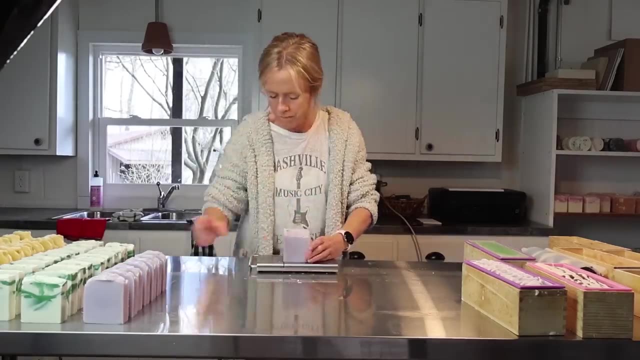 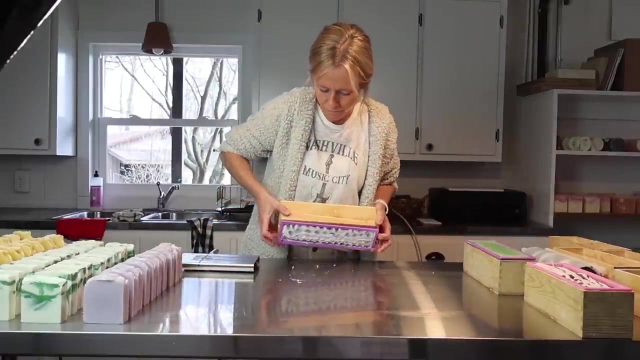 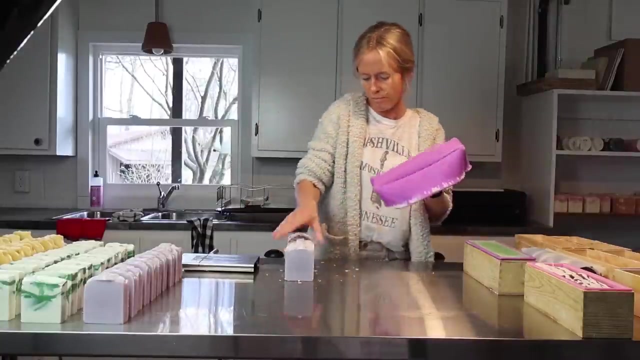 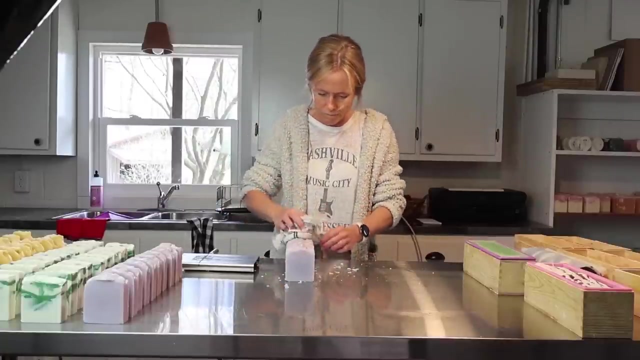 fairly. you know wipeable, like you can kind of wipe it off and it still looks pretty good. so if you're making like an automatic foreigner soap, that you're not the kind of one that's just a normal soap that you can wipe off and then you can start to clean yourself. 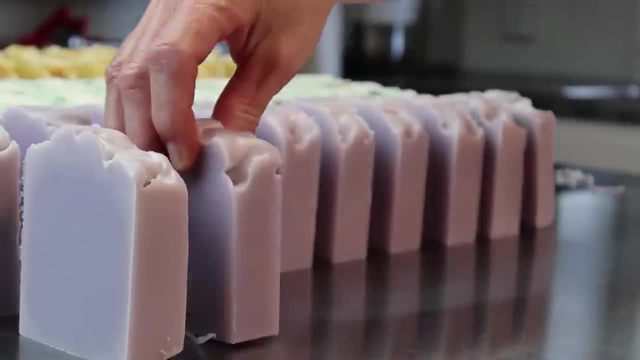 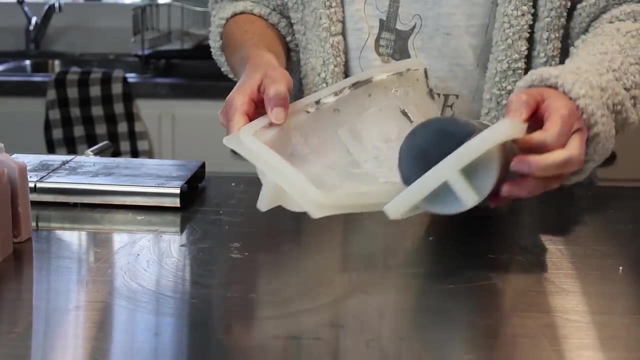 and then you can come back clean and try to clean yourself. so for me that's out of the question. and a couple other things I kind of forgot was the. the soap should have a bit of a blurring effect on what I'm using, but I don't know what that. 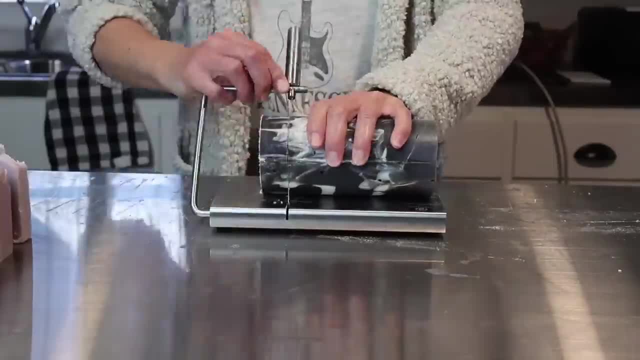 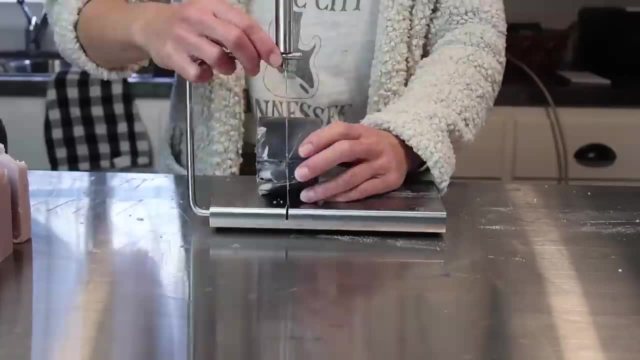 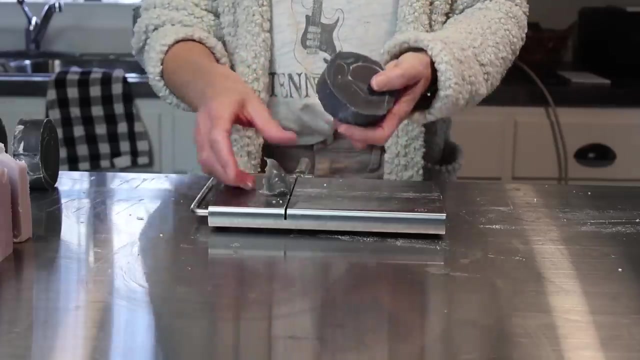 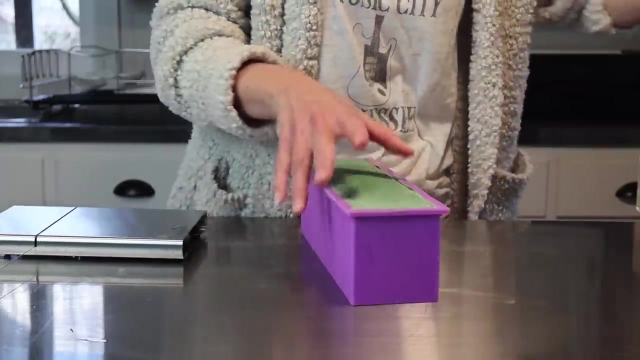 is because I'm not sure what that is. but I don't like the color of the soap because I don't know what that is. so I just keep going with it and I'll see if it works for some. so let's see how the grass soap turned out. actually, I'm kind of impressed. I. 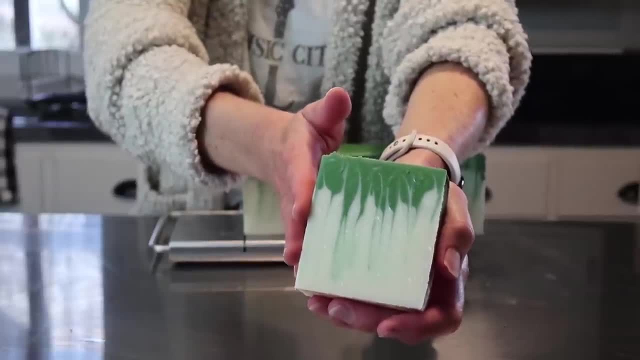 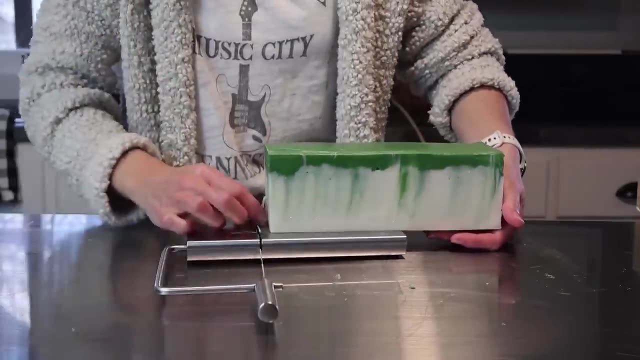 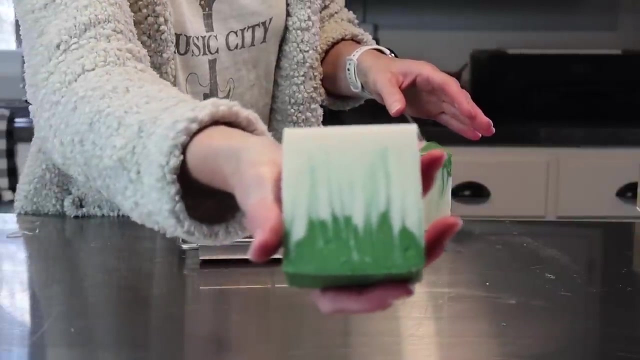 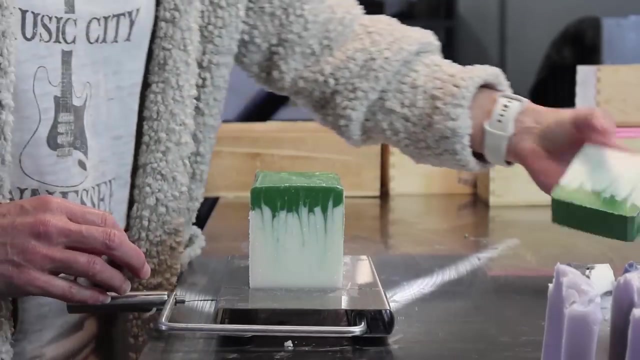 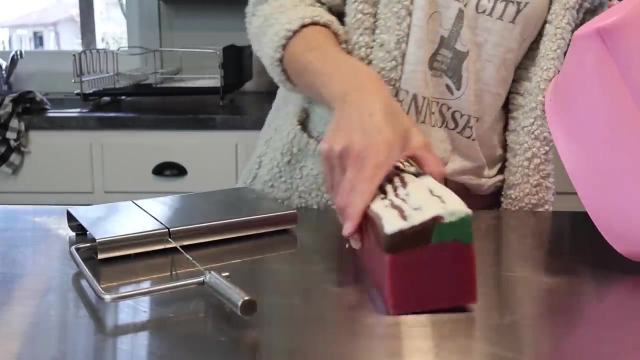 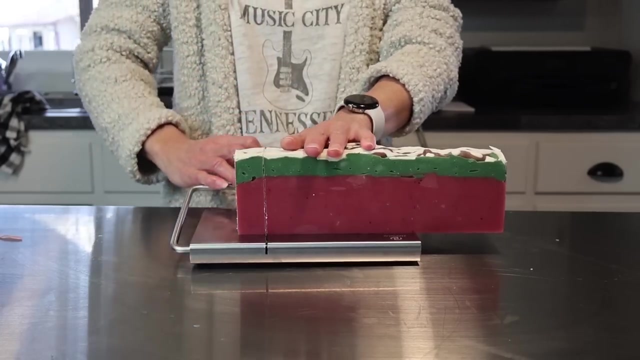 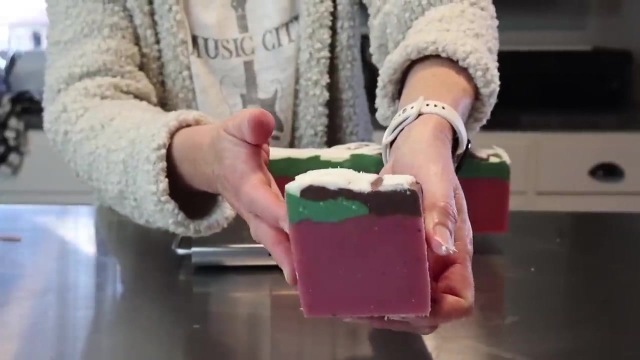 feel like it does look like blades of grass, and I might even end up turning it upside down, have the green at the bottom. that way it's more. you know grass like and appearance. I feel like this one might be the flop of the batch here, but at least I've tried it, I think. 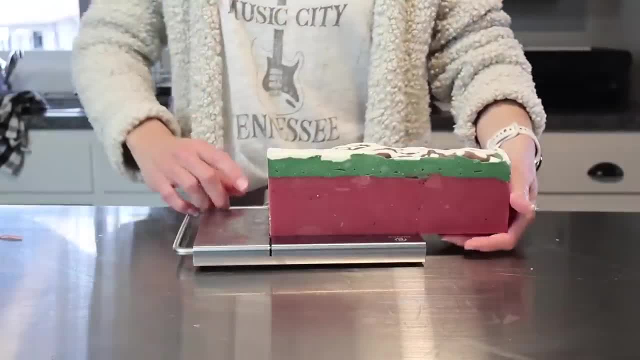 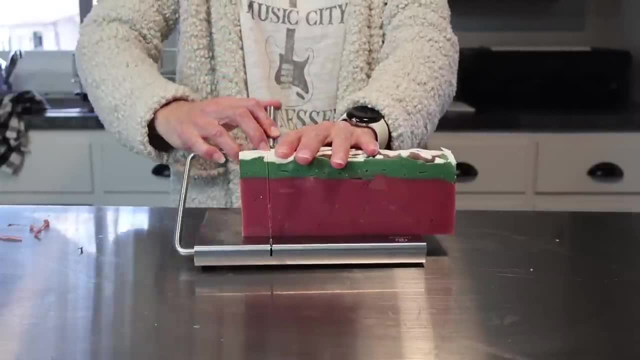 the colors need some adjusting if I were ever to do this again. like I mentioned, that green is too rich. I like a strawberry color. it even kind of looks like strawberry with those seeds in there. I'm already thinking: do I want to do a? you know, strawberries and cream maybe have just like a. 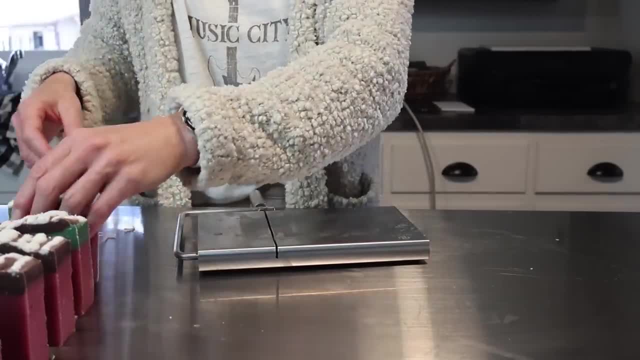 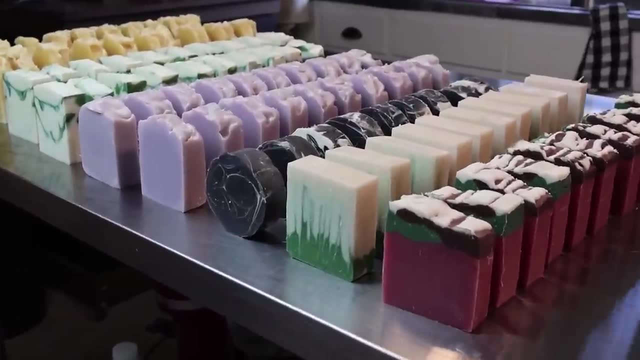 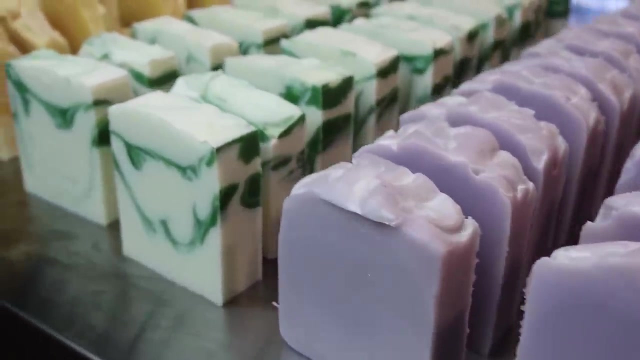 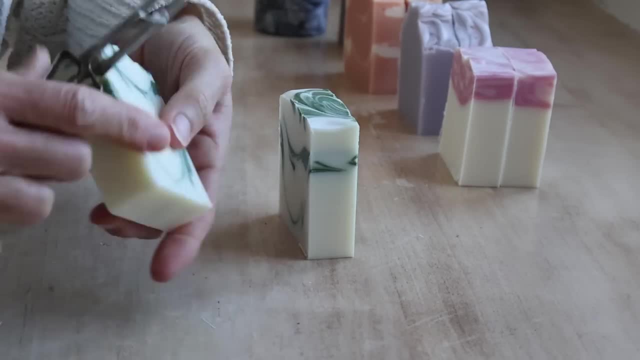 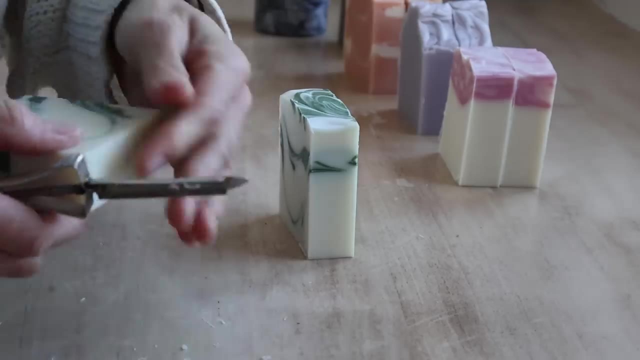 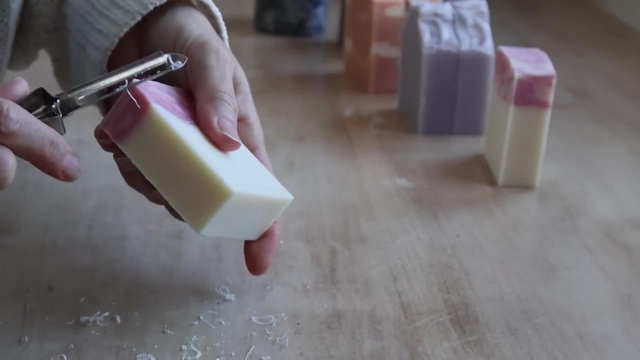 just to kind of clean it up a bit. of course, the soap I'm working on here is cured and ready to go. I'm not already shaving the one I just made. that will happen later. usually I do have a strawberry and lime scent here that smells amazing, and this one will be available on. 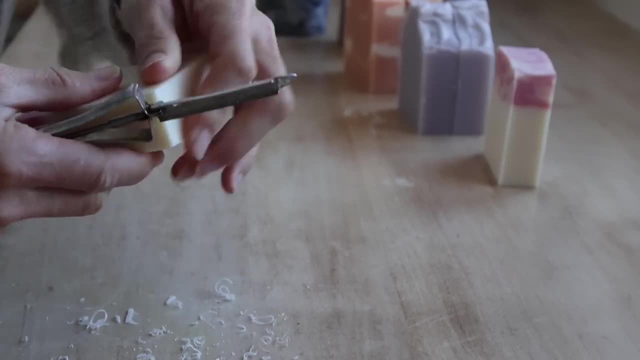 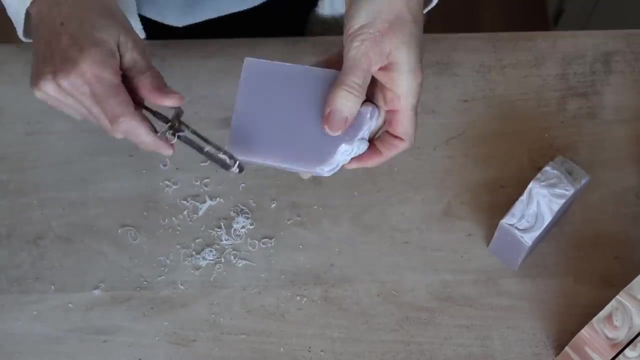 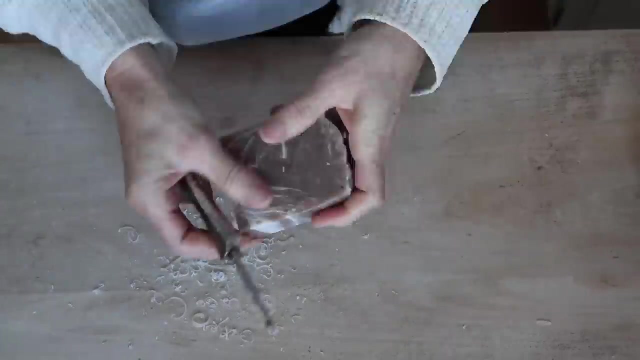 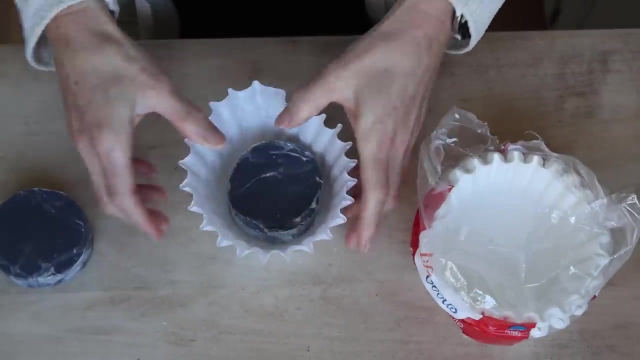 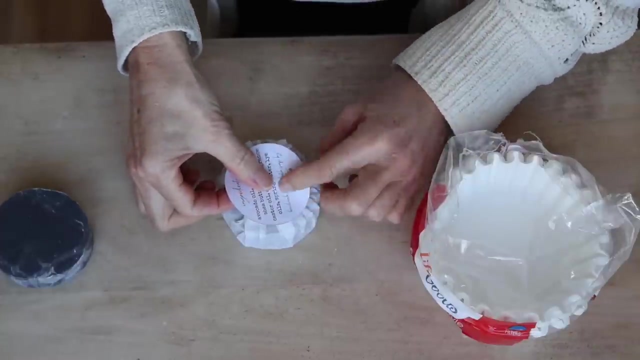 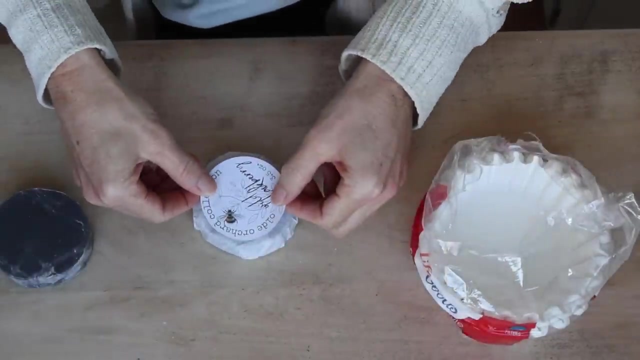 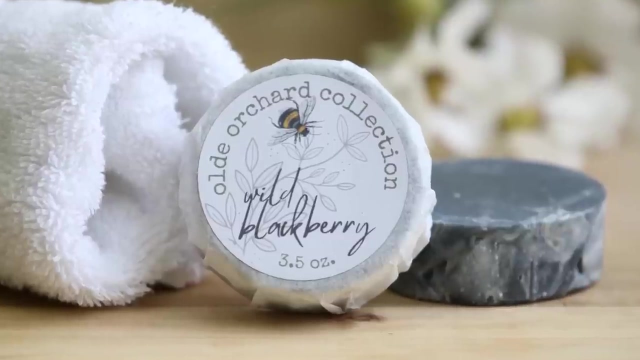 the Etsy shop, you're going to see a few other scents that I didn't make in this video but are going to be available, cured, ready to go. I saw on Pinterest how you can use coffee filters to wrap the soap, so I thought that would be so fitting for round soap. so that's how we're packaging these and I think at the point of filming here these might already be sold out. but stay tuned, we are going to have, you know, the one that I made here in this video that will be available in the next three to four weeks, and then I'm always making some more. so keep watch for that if you're wanting some of this cute old orchard collection soap. 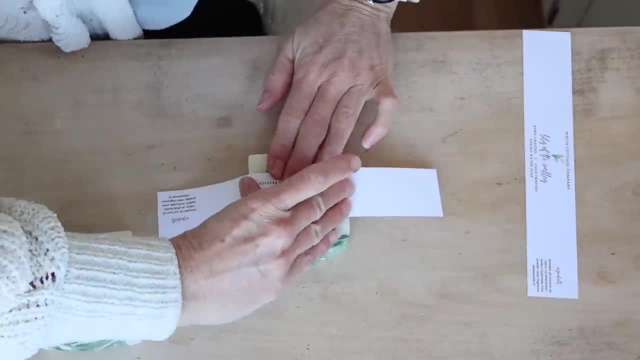 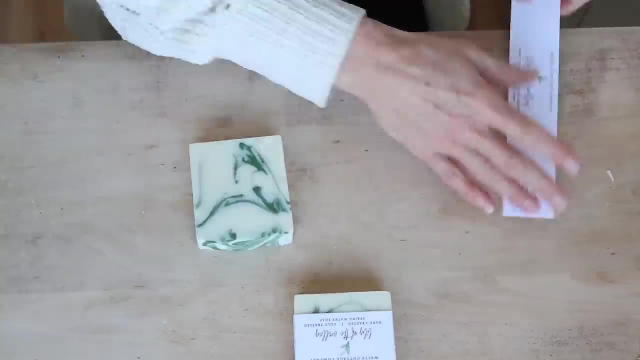 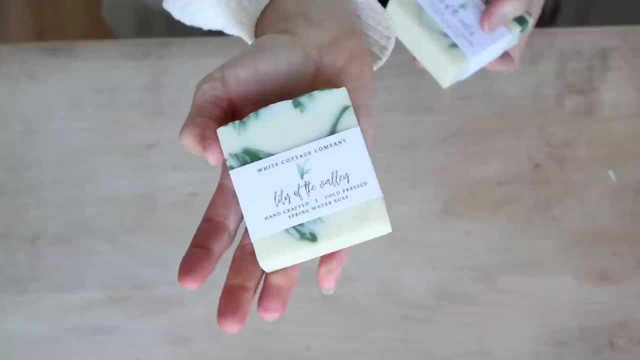 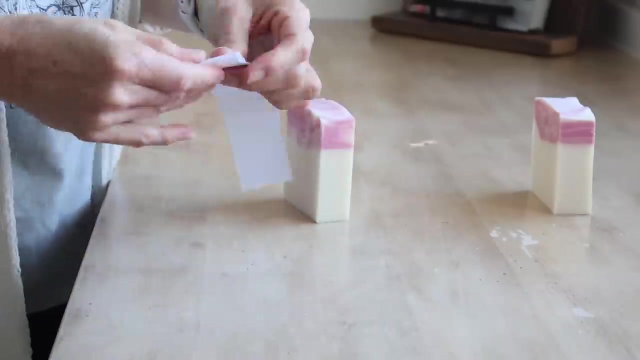 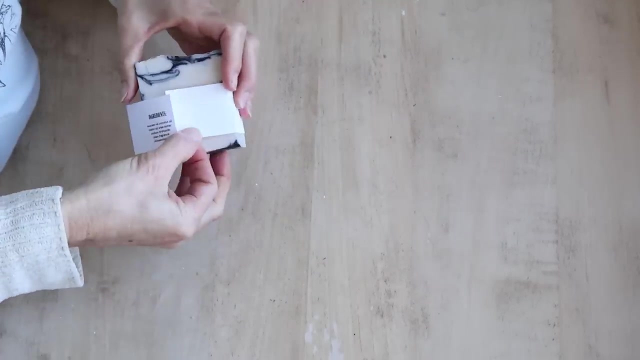 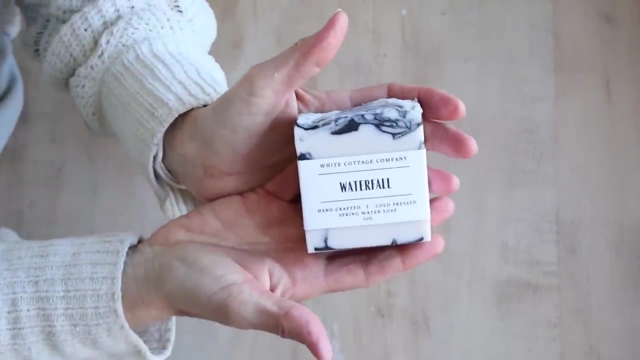 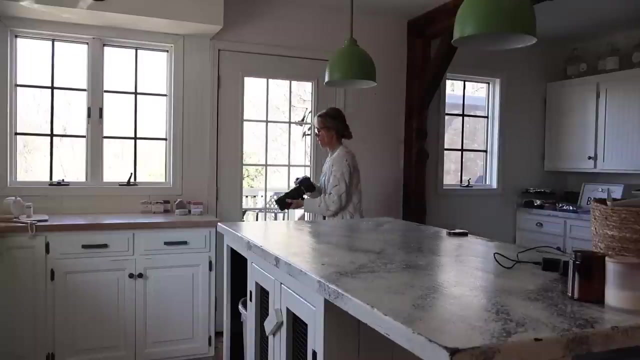 and I'll see you guys in the next video. bye, so one of the last steps, of course, is taking pictures of the soap, especially if we have new kinds, or sometimes I just like to take fresh, new pictures. I often do it right here on the kitchen countertop, where there's plenty of light. 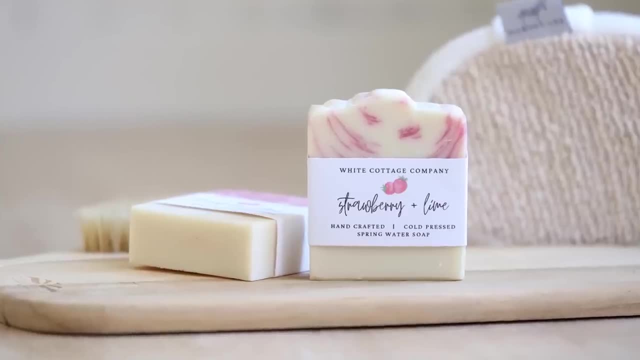 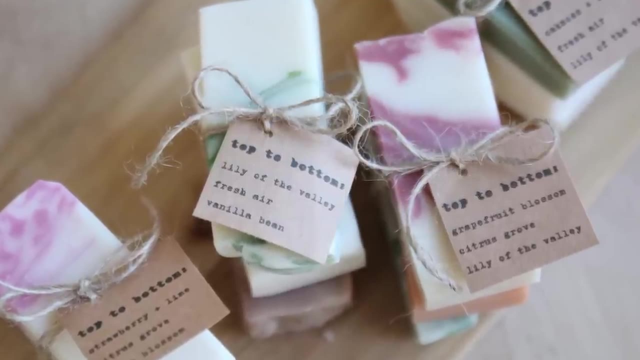 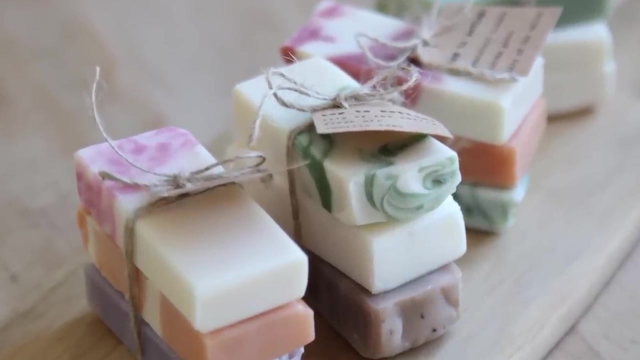 thanks for watching. we always have some soap ends and we package those kind of as a sample pack and at the point of filming here again, we might be out of them already. but keep a watch out for that listing in case we, you know, add some here in the next weeks.